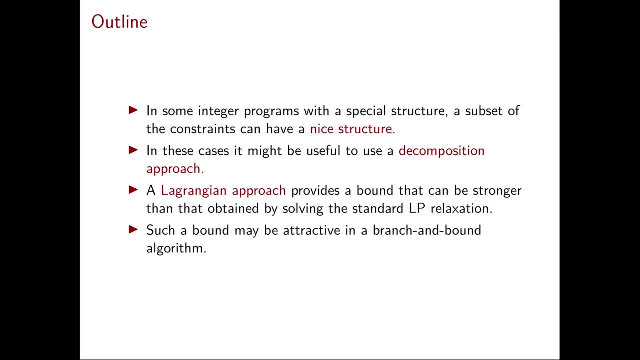 and you have a new part of the problem that complicates what you knew so far. In this chapter, we're going to discuss exactly how to approach these types of problems. In particular, we will discuss a Lagrangian approach which exploits the structure of the 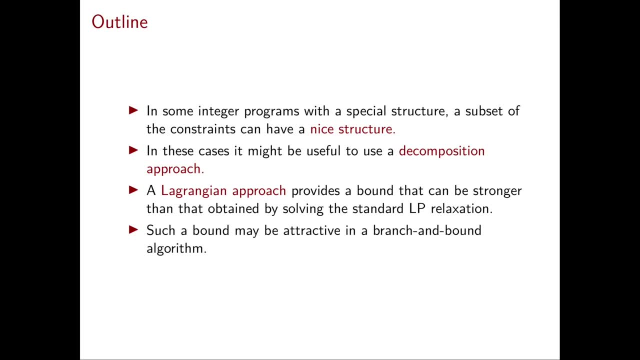 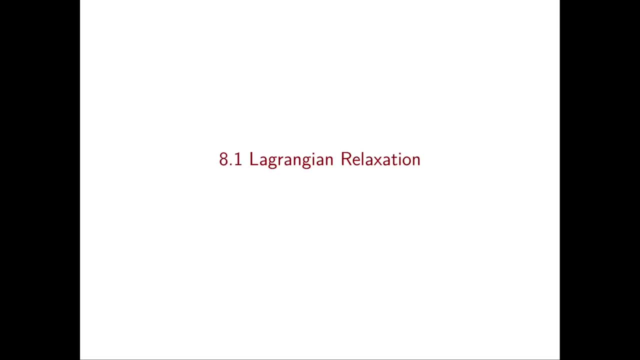 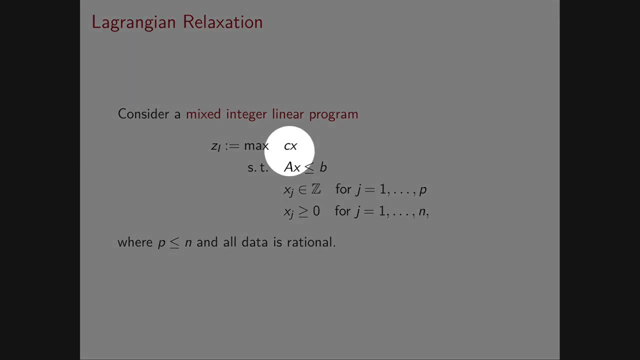 nice constraints to obtain bounds on your problem which are potentially better than those obtained with the standard LP relaxation. So let's start with the Lagrangian relaxation. Let's fix the notation for our mixed integer linear programming problem. In this problem we have n variables. 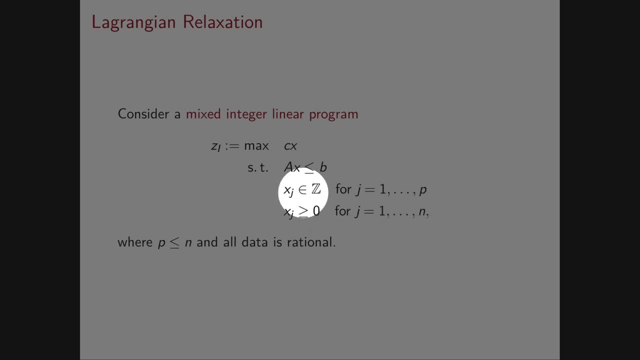 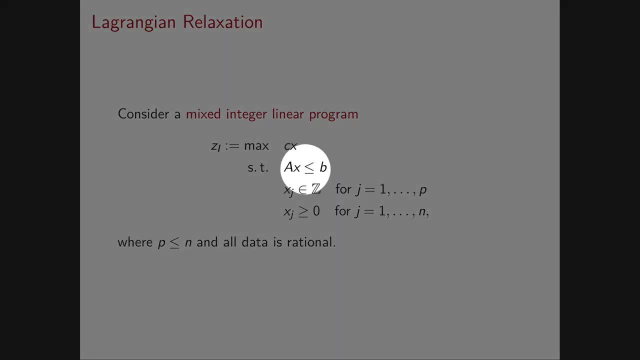 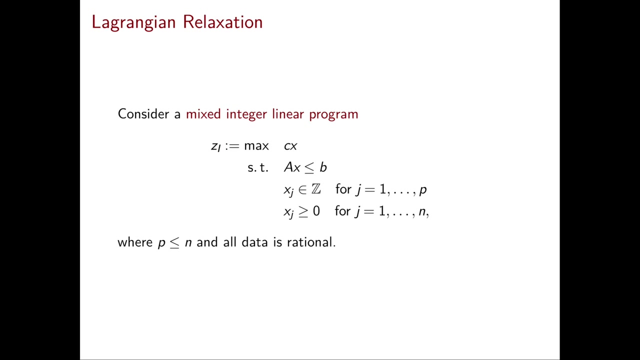 are required to be integer. Then we have a polyhedral region, ax, less than or equal to b, and we are maximizing an objective function, cx, and we denote by zi the optimal value of this integer program. Furthermore, we always assume, as always, that all the data is rational. 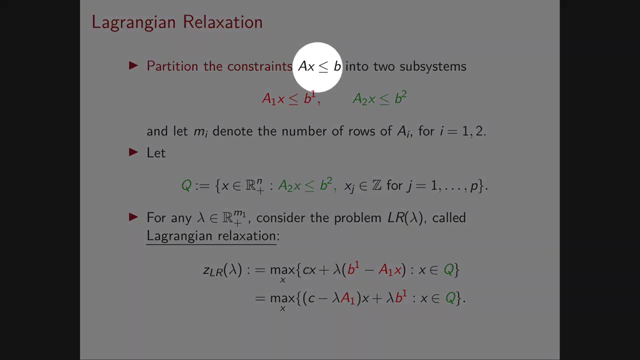 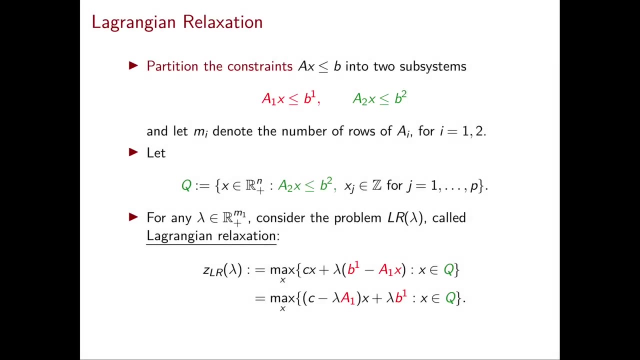 We immediately partition our inequality constraints into two subsystems, and we're always going to the note them by a1x less than or equal to b1, and a2x less than or equal to b2.. And we're also going to use mi to denote the number of rows of the matrix ai. This partition is, of course, up to us. We can. 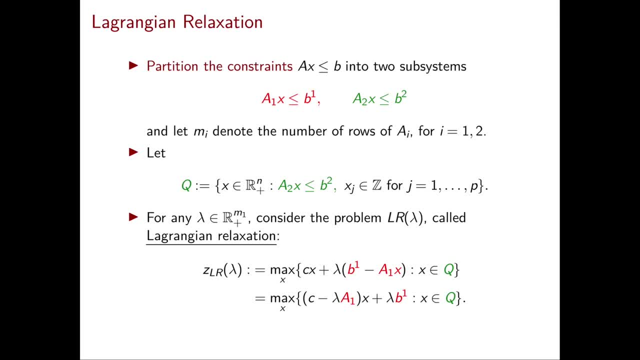 use any partition of this form and based on our partition. now I want to immediately define what is the Lagrangian relaxation. So the first thing I need to do is define the following mixed integer linear set: It is essentially the mixed integer linear set of our original problem, but where we 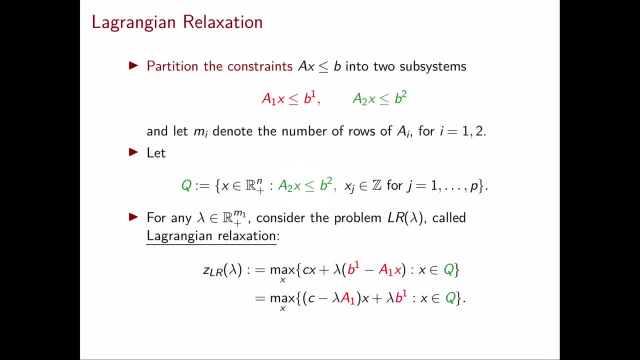 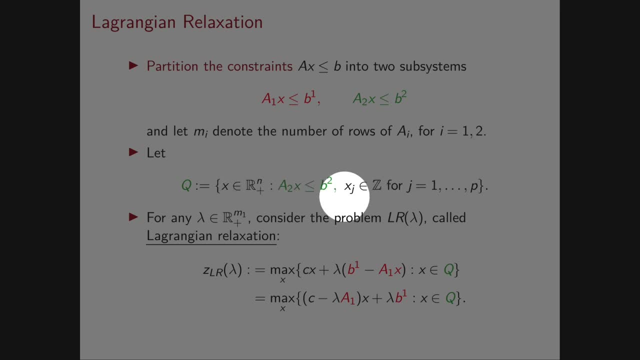 drop the inequality constraints of the red system. So, as you can see, we have non-negativity on all the n variables, we have integrality on all the first p and then we only have the constraints in green. We're now ready to define the Lagrangian relaxation. Pick any lambda in R plus m1. 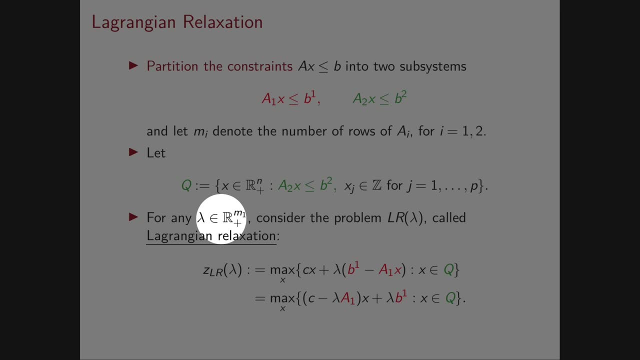 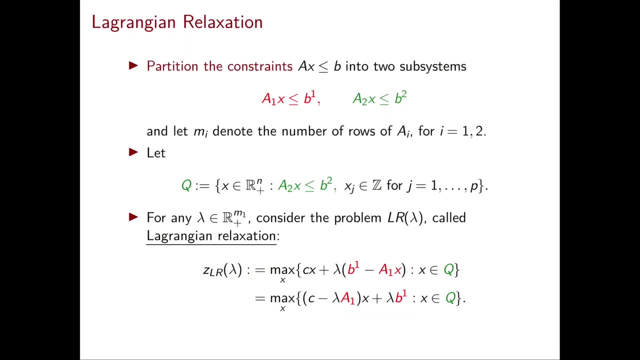 So this is a vector of multipliers associated with an integer with the red constraints. then we define the Lagrangian relaxation- and it's always denoted as LR- of lambda, because of course it depends on your choice of lambda, and it's defined as follows: you want to maximize over the set Q that we 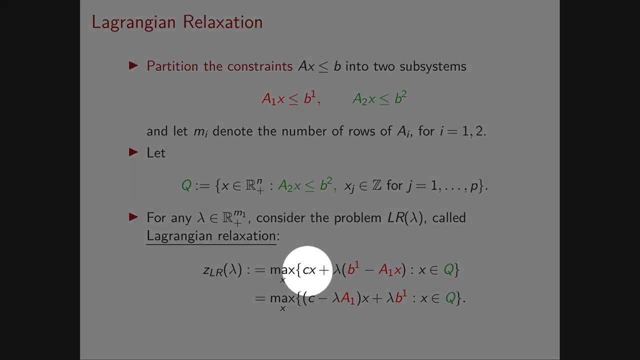 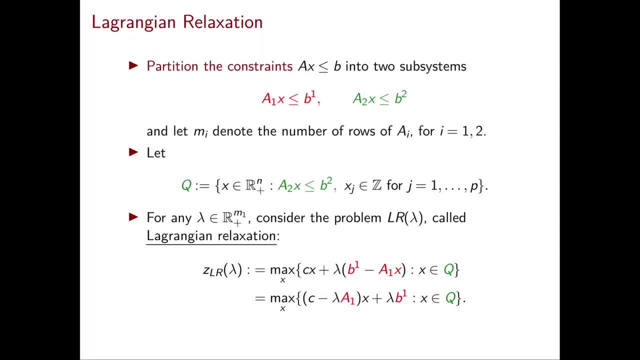 just defined and your objective function is the original CX. but since in Q we no longer have the red constraints, we are somehow adding those inequalities in the objective function as a penalty in particular. the objective is then CX plus lambda d1 minus a1 X. so this is our definition and I just want to give you a 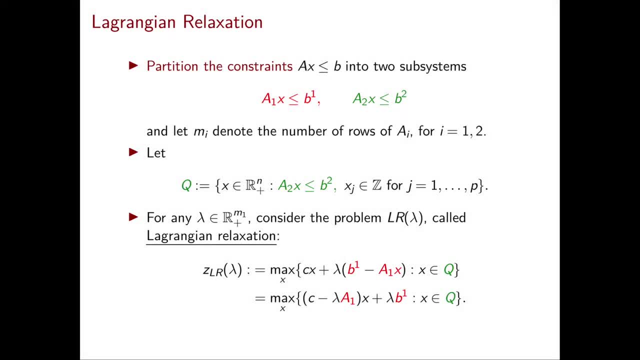 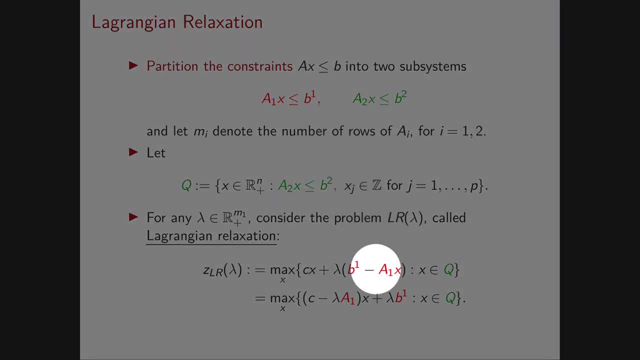 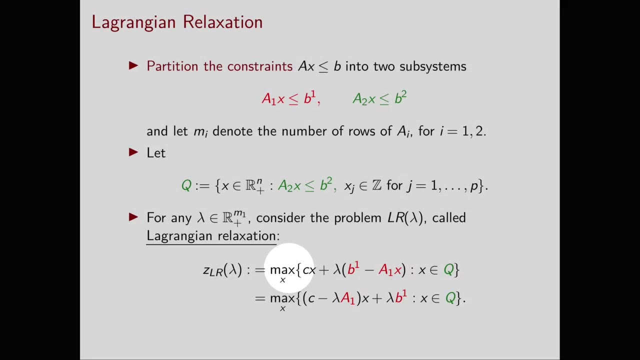 little bit the intuition behind this. the idea is that if you do not satisfy the red constraints, then this quantity is negative and And since lambda is non-negative, this whole part of the objective is negative, and so it drives down our objective function, making it far from optimal, since we're maximizing. 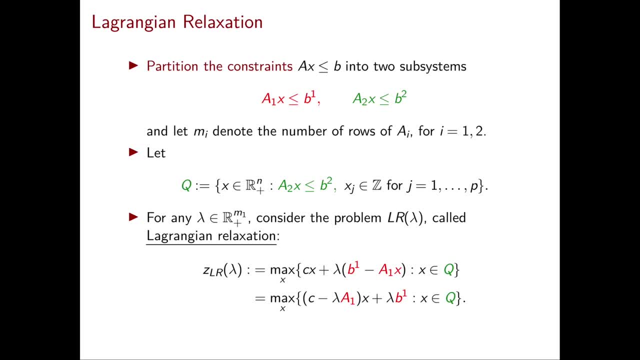 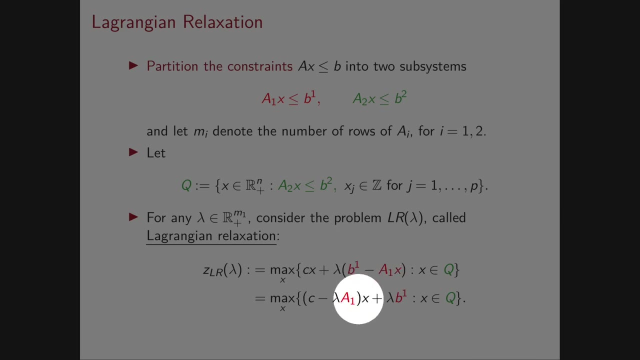 Now, the optimal value of this maximization problem is denoted by ZLR of lambda, And here, in the last line, we simply have the same Lagrangian relaxation, just rewritten in a way where the x variables are all together, so that it's a bit clearer what is the function that you're maximizing. 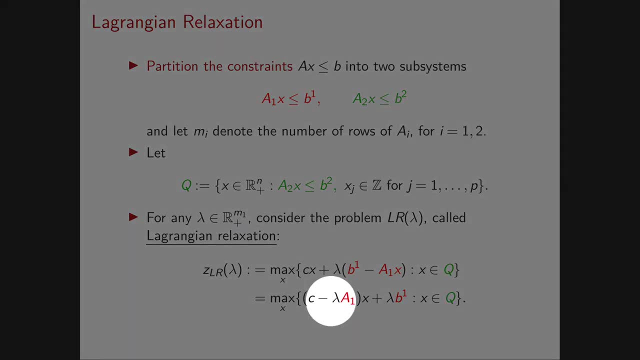 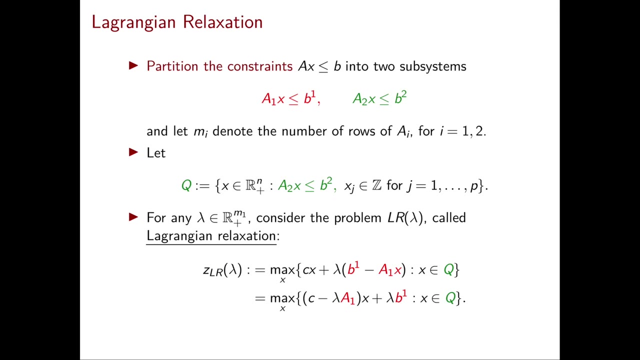 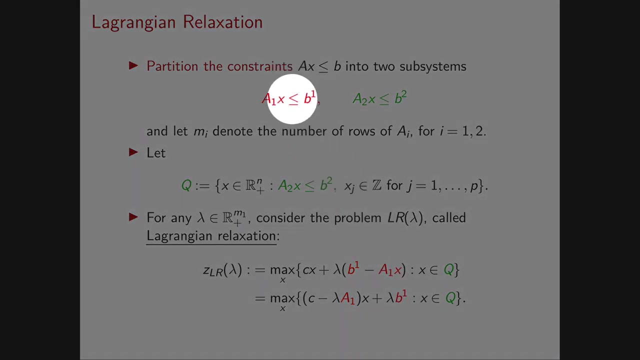 In fact such objective function is C minus lambda A1 times x, because essentially lambda B1 is a constant once you have fixed your lambda. So the definition we gave of Lagrangian relaxation applies to any partition of AX less than or equal to B. 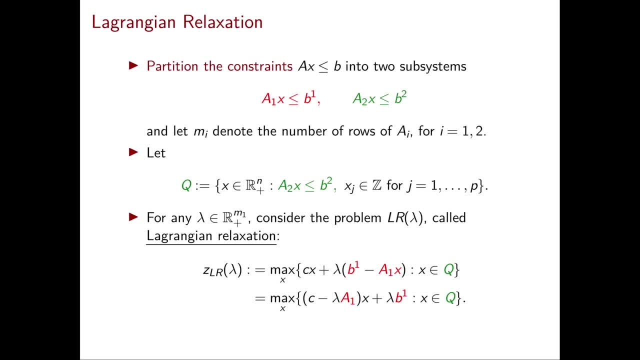 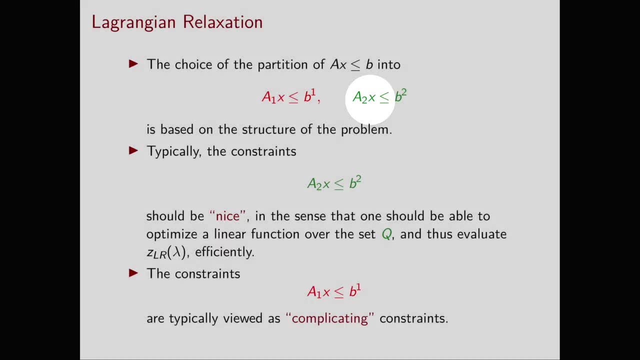 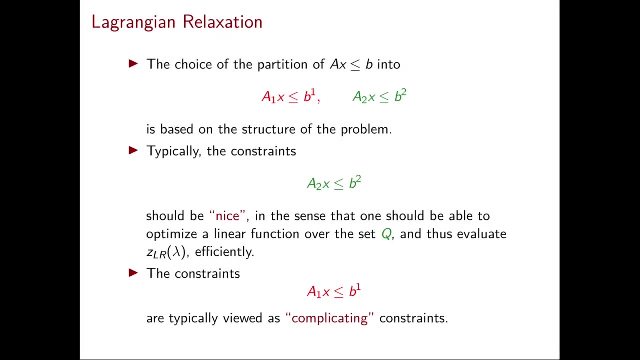 in red and blue. However, in practice, how should you subdivide your system into these two subsystems? Well, typically, the green constraints, as the color suggests, are nice constraints in the sense that you are able to optimize any linear function over the set Q. 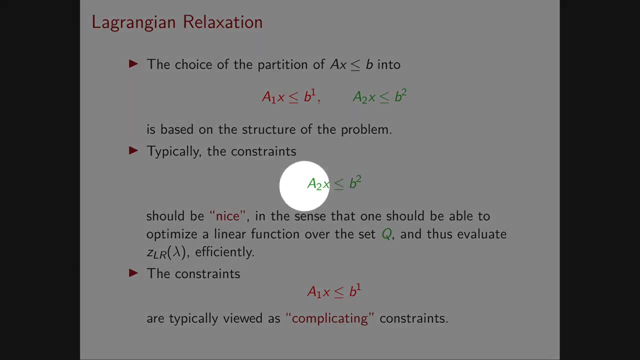 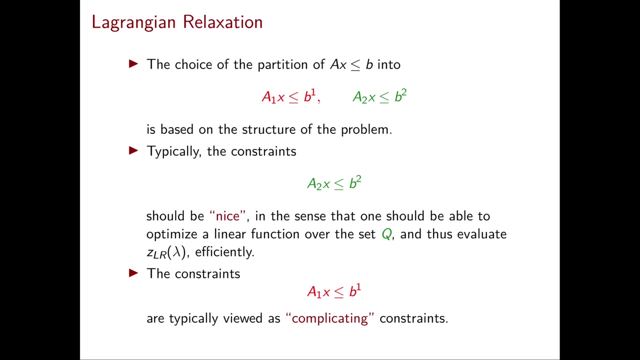 which includes only these constraints. In fact, this allows you to evaluate ZLR lambda efficiently for any lambda, Therefore, the red constraints are viewed as the complicated constraints. So essentially, these are the constraints that you need to remove from your mixed integer linear set. 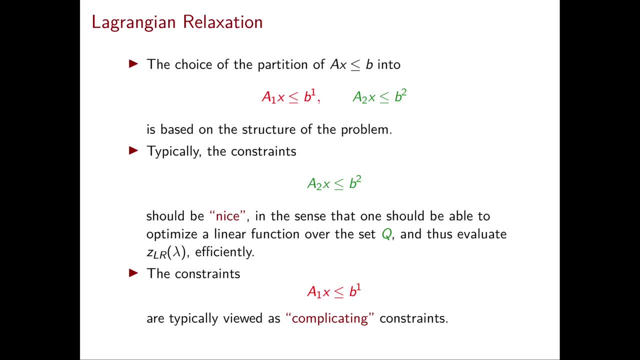 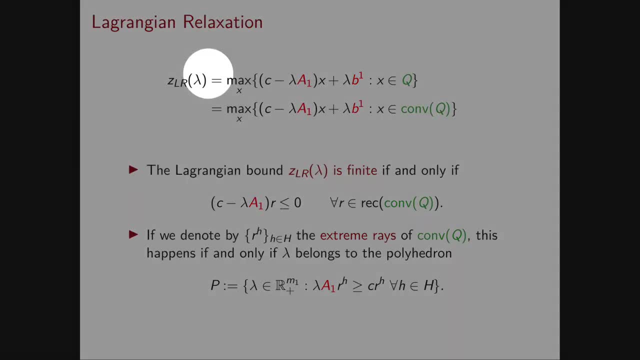 so that you can optimize over it efficiently. Now let us discuss a little bit the Lagrangian relaxation from a polyhedral perspective. In the first line here I have our definition of Lagrangian relaxation that we just saw a couple of slides ago. 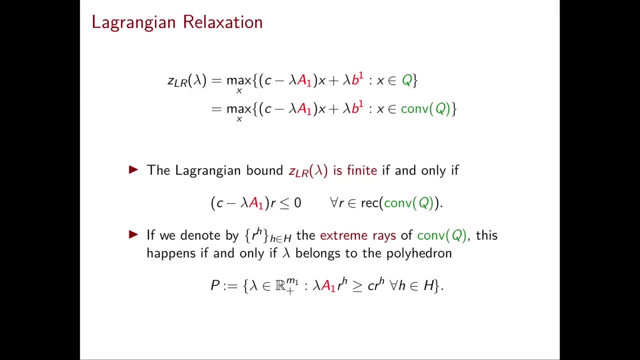 We know very well that optimizing a linear function over a mixinteger linear set is the same as optimizing it over its convex hull. Therefore, the Lagrangian relaxation could be solved in principle by solving just this LP, if we knew the convex hull of Q. 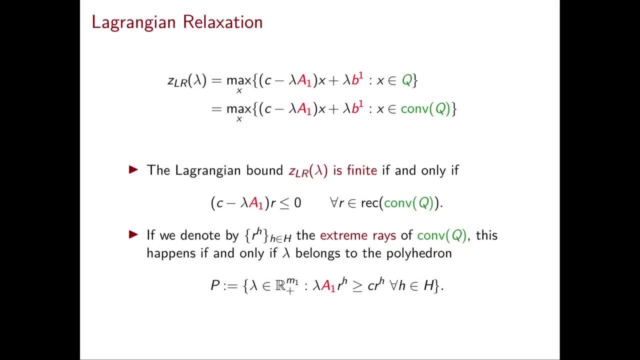 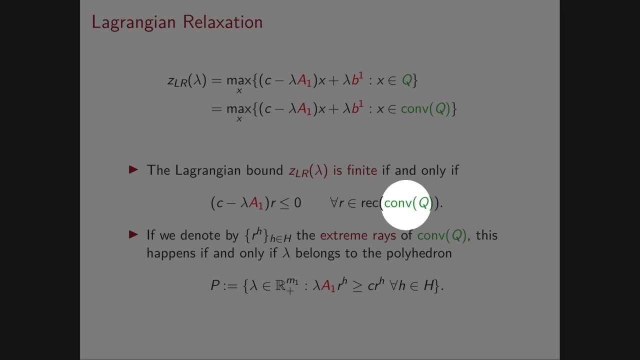 But now we can analyze a little bit better the Lagrangian relaxation, polyhidrally. In fact, we immediately understand that the objective value of the Lagrangian relaxation is finite, if and only if, for every ray of the recession cone of the convex hull of Q. 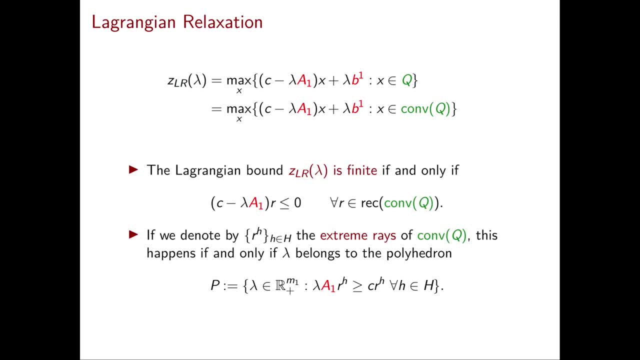 we have that along that ray the objective function decreases. In formula we look at our objective function and evaluate it on the rays C minus lambda, A1 times R must be less than or equal to zero, because otherwise, if it's greater than or equal to zero, you can travel along that ray. 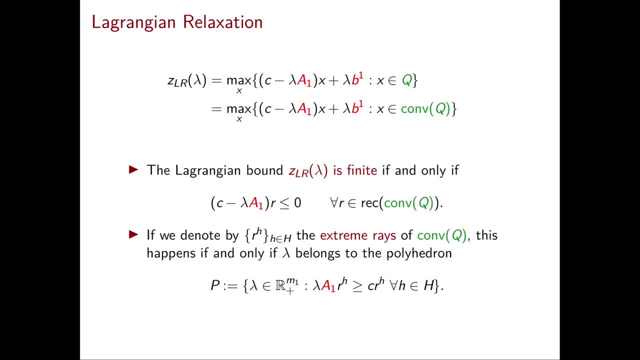 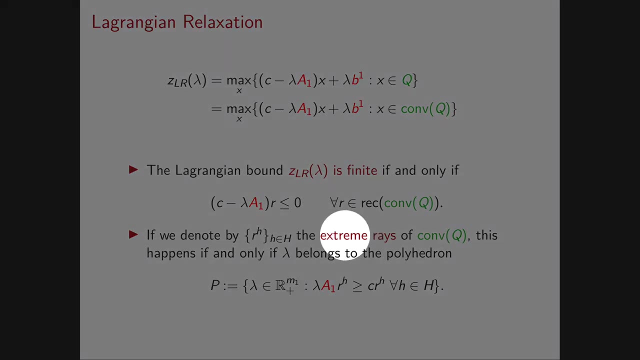 and your objective can always go to plus infinity, since you're maximizing In particular. now let's look instead at the extreme rays of the convex hull of Q, Then Z, L, R. lambda is finite if, and only if, for every such extreme ray, this condition holds. 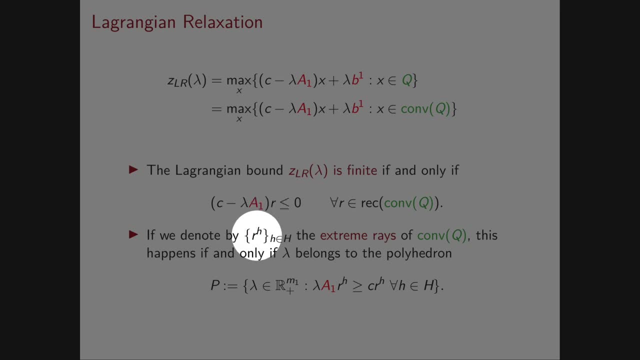 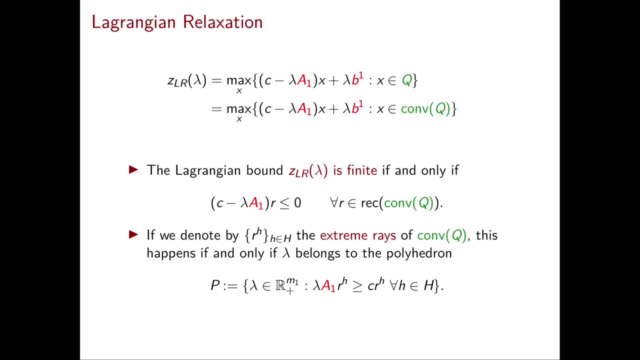 So if we substitute in this formula R to be one of these R H, we obtain exactly this inequality, which must hold for every extreme ray. Therefore, the Lagrangian bound is finite if, and only if, our non-negative multiplier lambda satisfies all these inequalities. 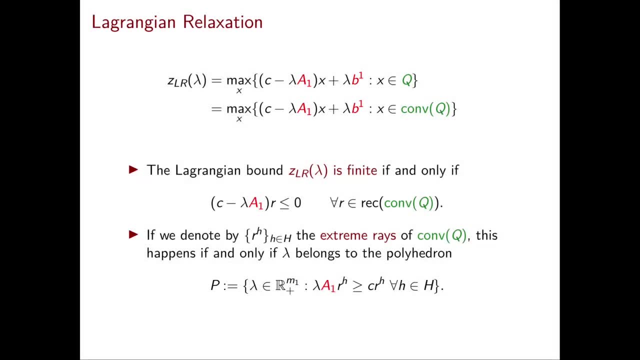 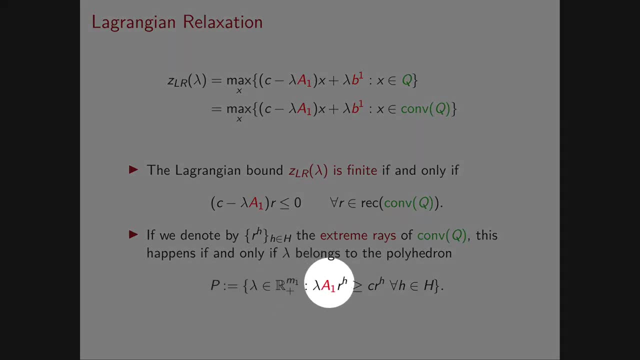 And we're going to denote this polyhedron by a capital, P. Note that in this description the variables are just lambda. Everything else is data, So A1,, of course, is data. R H is just an extreme ray of the convex hull of Q, so it's data. 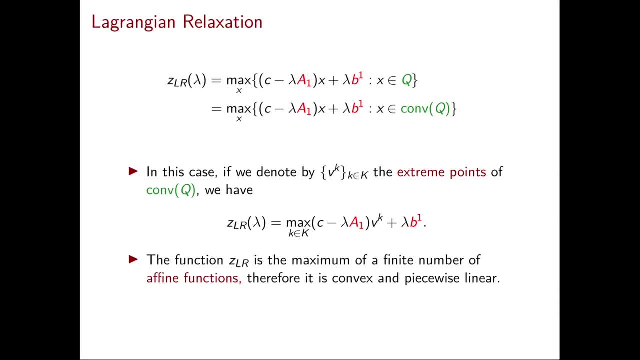 And same goes for C. So now assume that we satisfy these conditions. In this case the Lagrangian bound is finite. Then what is actually the value of this Lagrangian bound? Well then, it must be the maximum of our objective function. 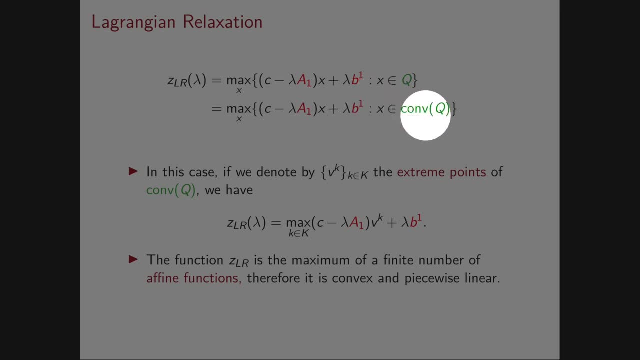 over all the vertices of the Lagrangian bound. That is the maximum of the polyhedron conv Q. So denote by VK all the extreme points of conv Q. Then the Lagrangian bound is the maximum of the objective function evaluated in the vertices. 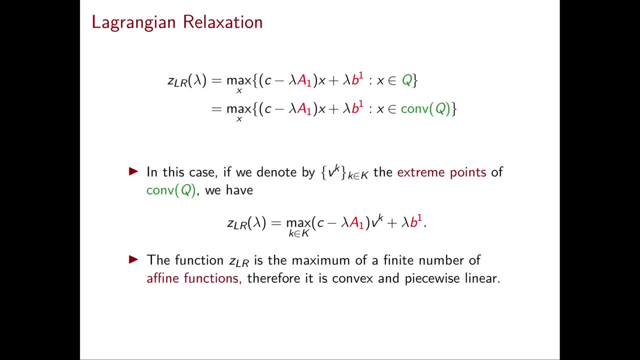 plus lambda B1, which is just our constant in the objective function. And finally, this formula allows us to understand a little bit better how this function Z L R of lambda looks like. In fact, it is the maximum of a finite number of affine functions. 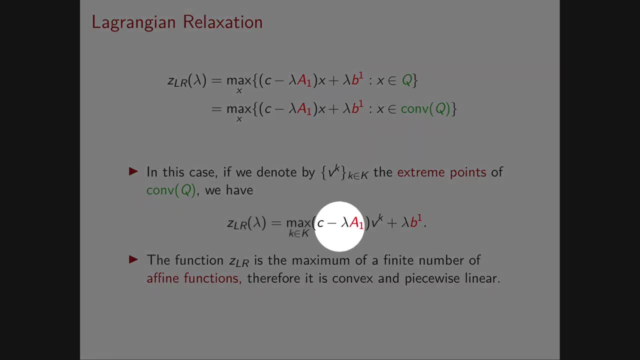 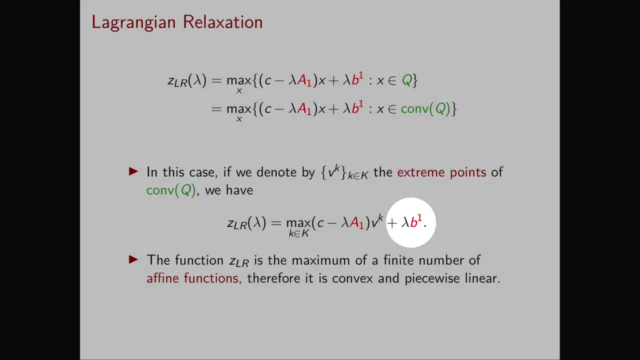 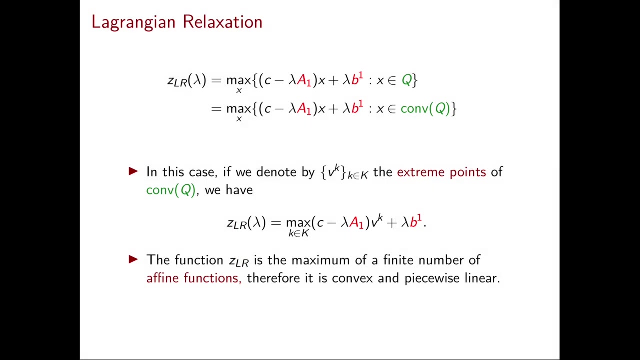 namely the function C minus lambda A1 times VK plus lambda B1.. These are all affine functions of the variable lambda. In fact, both this term and this term is linear in lambda And plus you have C, VK, which is a constant. 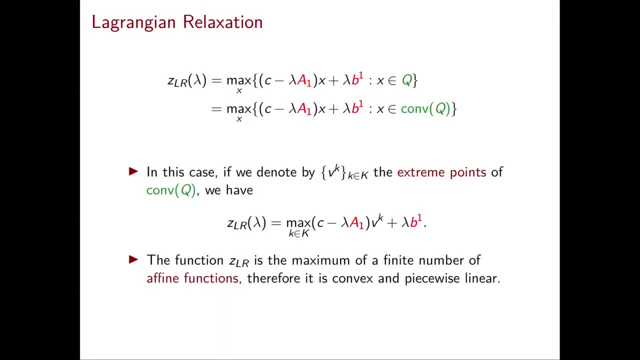 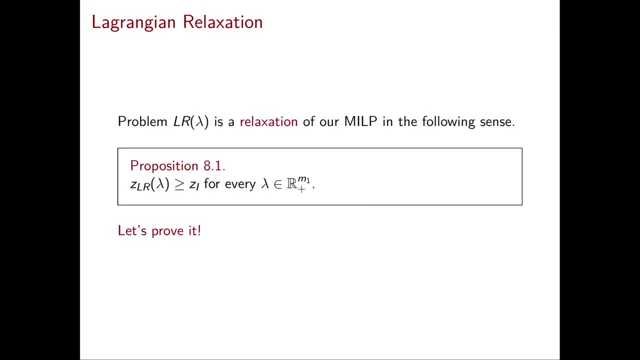 Now you're taking the max of all these affine functions, And so, as we have seen in chapter two, this is a convex and piecewise linear function. The next proposition implies that the Lagrangian relaxation allows us to bound our optimal value of the original integer programming problem. 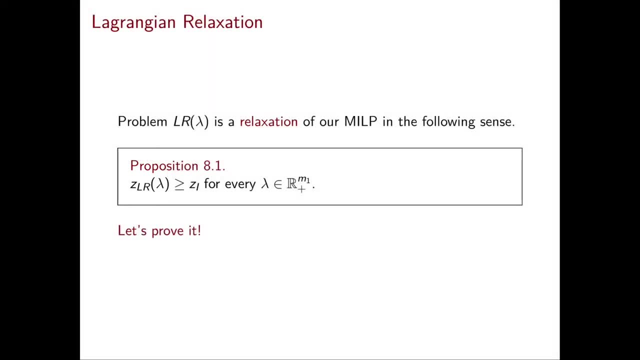 In fact, this proposition says that the Lagrangian bound is greater than or equal to Z I for every lambda. Let's now prove this proposition. The first thing to observe is that we can assume that a feasible solution of the mixed integer linear programming problem exists. 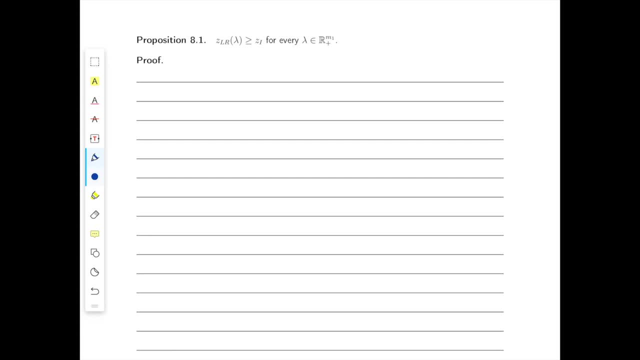 because otherwise we have Z I equal to minus infinity, And so of course the Lagrangian bound cannot be smaller than that, So obvious when Z I is equal to minus infinity. So we assume that a feasible solution of the original mixed integer linear programming problem exists. 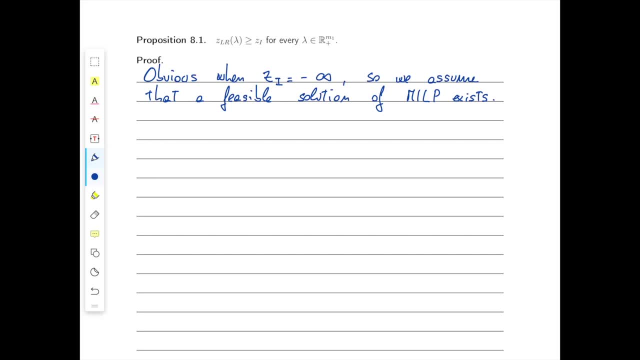 So how are we going to show this proposition? We pick any feasible solution of the mixed integer linear programming problem. We show that it's also feasible for the Lagrangian relaxation and that it has objective value greater than or equal to its original objective value. 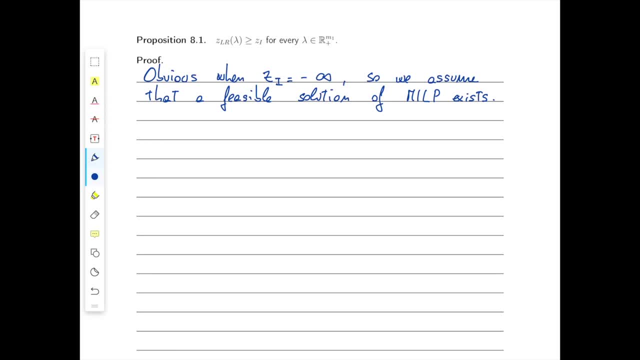 That's enough to prove that the Lagrangian bound is at least Z. I So let X bar be any feasible solution of the mixed integer linear programming problem. Well, so we know that X bar is in Q, since Q is a relaxation of the mixed integer linear set. 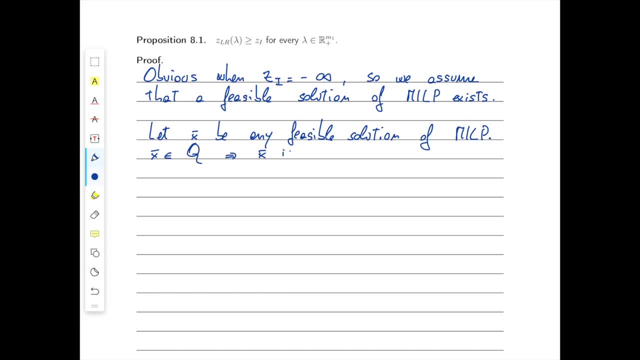 of the original problem. Therefore, X bar is a feasible solution of the Lagrangian relaxation with multiplier lambda. Now the objective value of X bar in the Lagrangian relaxation is just, by definition, CX bar plus lambda times B1 minus A1X bar. 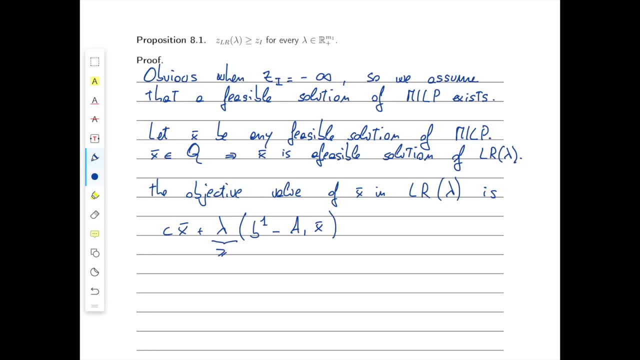 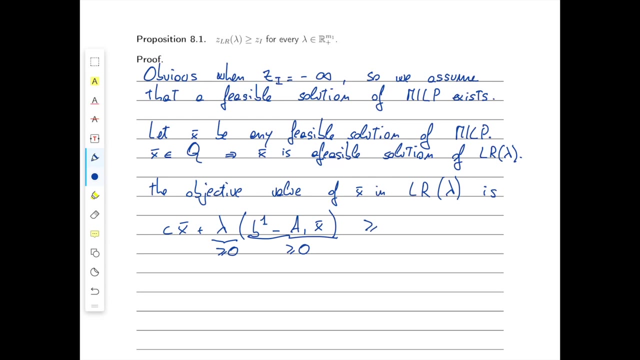 Now lambda is by definition greater than or equal to zero, And since X bar is feasible for the original program, we also have that A1 minus A1X is greater than or equal to zero. So this objective value is greater than or equal to CX bar. 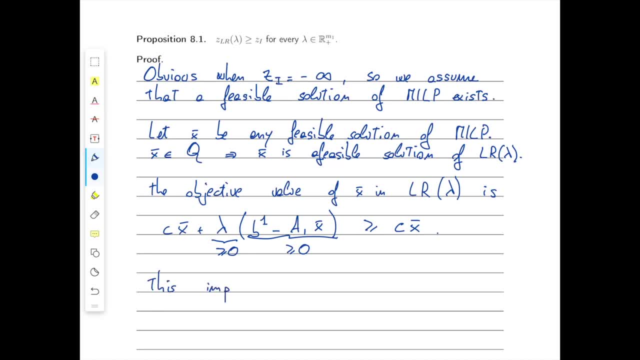 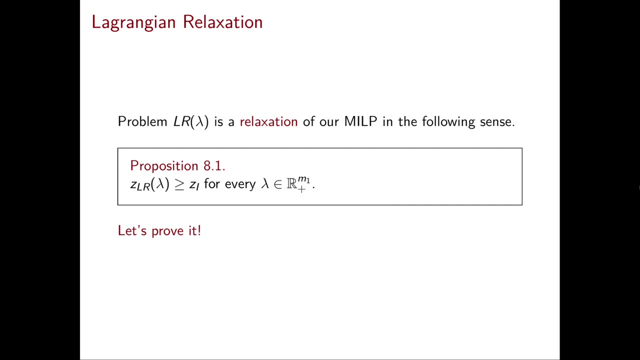 So this implies that the Lagrangian bound is greater than or equal to Z I, And that's the end of our proof. So let's get back to the slides. So far we have defined the Lagrangian relaxation for any non-negative lambda. 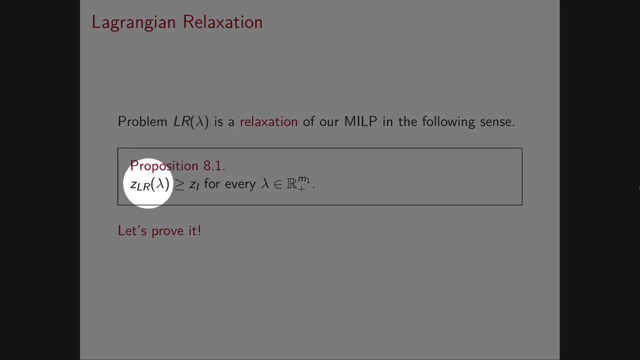 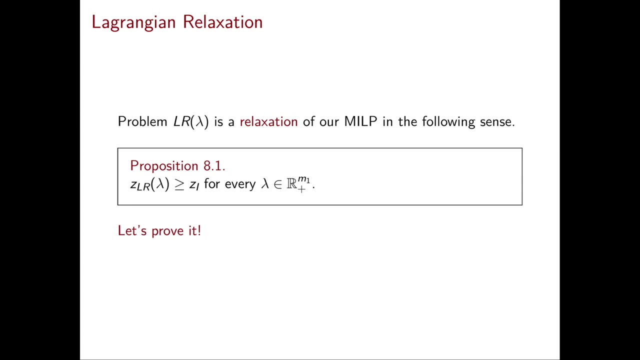 And each one of these Lagrangian relaxations gives us an upper bound on Z I. So it's only natural to ask what is the best upper bound that we can get, meaning, of course, the smallest upper bound that we can obtain. 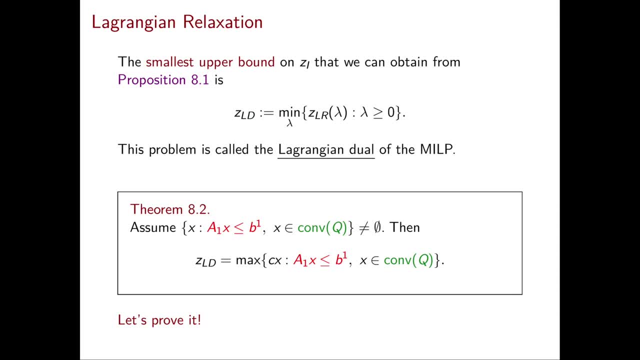 And this leads us to the definition of Lagrangian dual, which is defined as the minimum Lagrangian bound for any lambda greater than or equal to zero. While the optimization problem is called the Lagrangian dual, the corresponding optimum objective value is denoted by ZLD. 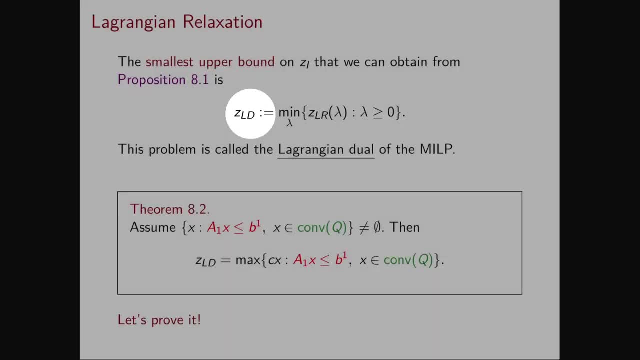 The next theorem characterizes ZLD as an optimal solution to a linear programming problem. In fact, it says that ZLD is the maximum of the original objective function CX over the convex hull of Q, intersected with the complicating constraints in red, Provided that the corresponding polyhedron 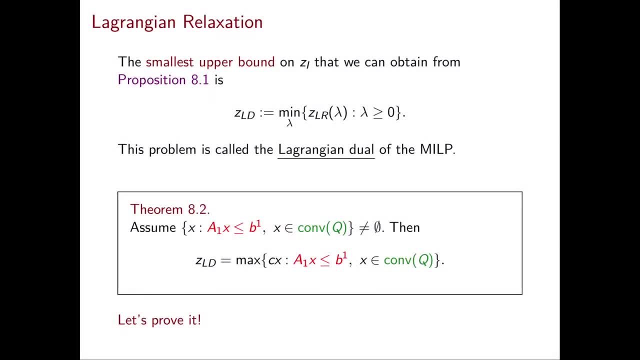 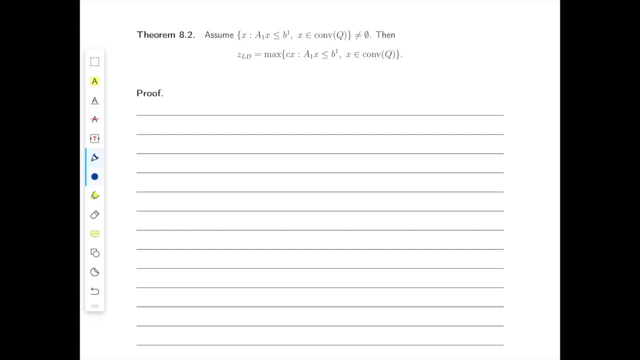 which is the feasible region of this linear optimization problem, is non-empty. Now let's prove this theorem. How can we prove this theorem? So let's look at the statement for a second. So we want to show that the Lagrangian dual 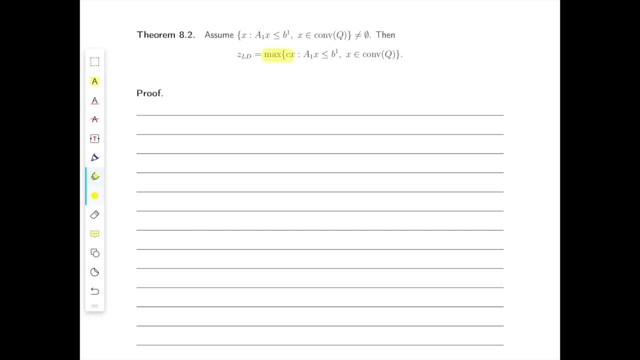 is equal to this linear programming problem in maximization form. As the name suggests, we're going to use duality to prove this theorem. Now, the dual of a maximization problem is a minimization problem, of course. So if ZLD was a minimization problem, 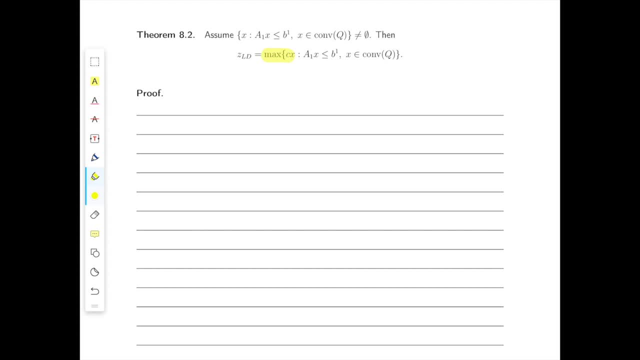 we would be somewhat happy because then we could take the dual and hope that it's actually this maximization problem. in the statement, However, note that ZLD is not, in its current form, a minimization problem. In fact, it is defined as the. 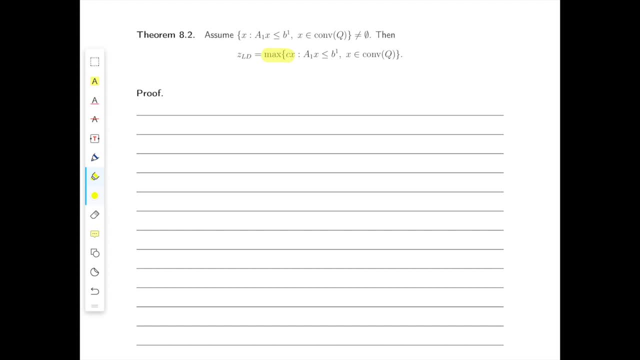 minimum of all the Lagrangian relaxations, and each one is a maximization problem. So, in order to obtain that ZLD is a minimization problem, we're going to transform every Lagrangian relaxation as a minimization problem so that ZLD. 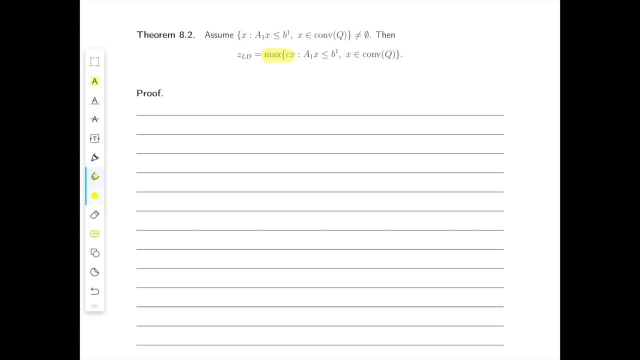 instead of being a min-max problem, will be a minimization problem. So since we're always working with the convex hull of Q and we want to use essentially linear programming, the first thing we want to do is introduce a notation for such a convex hull of Q. 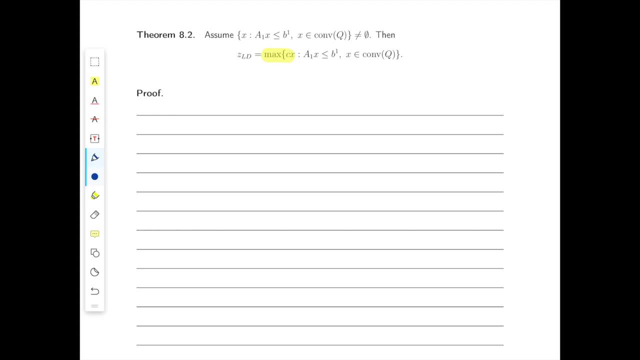 as a matter of linear inequalities, which we can do by Mayer's theorem. So let's do that. Since a2x less than or equal to b2 is a rational system by Mayer's theorem, there exists a system: Cx less than or equal to d. 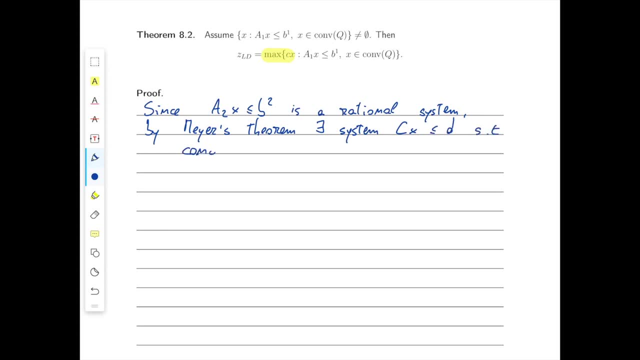 such that the convex hull of Q is the set of points in Rn, such that Cx less than or equal to d Great. Now let's write our Lagrangian relaxation in minimization form. So for every lambda greater than or equal to 0. 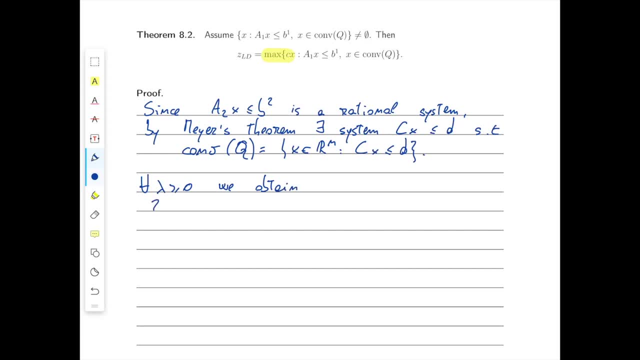 we obtain ZLD, LR lambda is equal to so by definition. it's the maximization problem with objective C minus lambda A1x, plus lambda B1 over the convex hull of Q, which we then write as Cx, less than or equal to d. 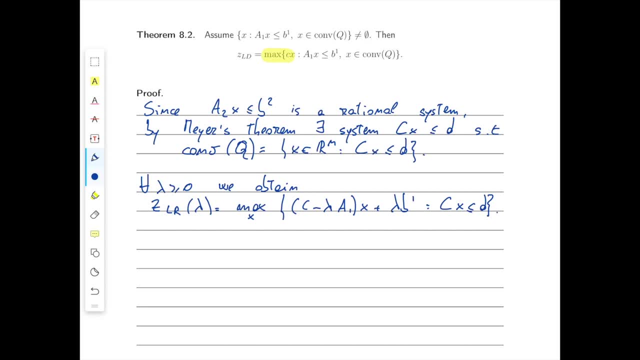 So now this definitely looks like a linear programming problem, so we can take the dual. So this is the min over variables mu Of mu d plus lambda B1, such that mu C equal to C minus lambda A1 and mu greater than or equal to 0. 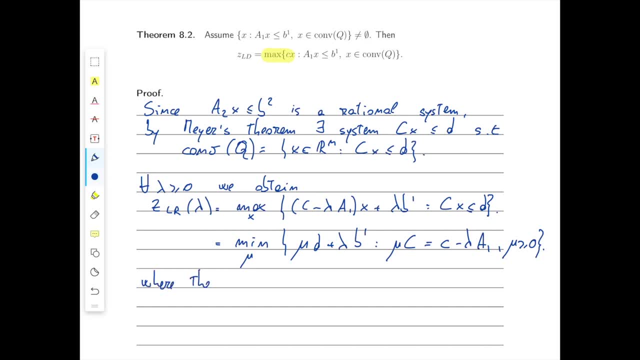 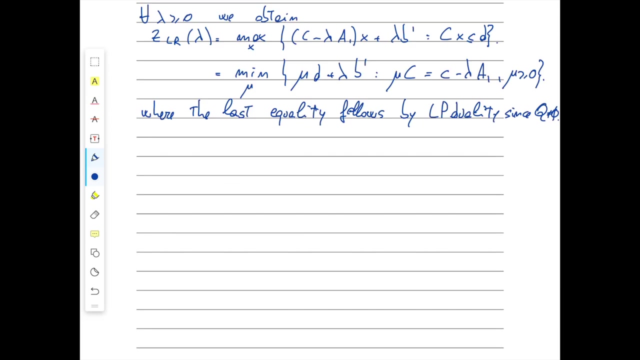 where the last equality follows by Lp duality. since Q is not empty, At this point we can finally write our ZLD, our Lagrangian dual, as a pure minimization problem. So follows that ZLD is equal. so by definition, 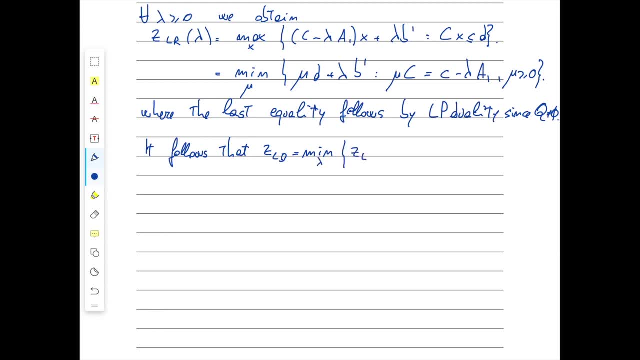 it's the minimization problem over lambda of ZLR lambda for every lambda greater than or equal to 0.. So now it is the minimum over lambda and mu of mu d plus lambda B1, such that lambda A1 plus mu C equal to C. 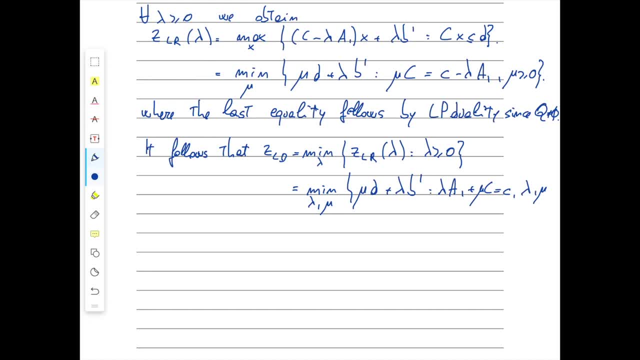 lambda mu greater than or equal to 0.. Let's take the dual As we discussed. the latter is the dual of the Lp max, Cx with A1x less than or equal to B1 and Cx with A1x less than or equal to B1. 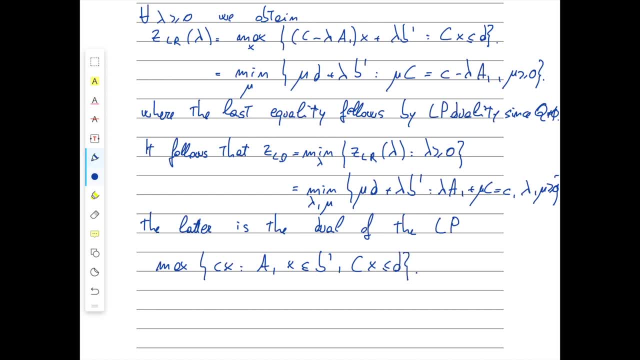 and Cx less than or equal to D. And we're done. So there optimal values coincide because the primal is feasible by assumption, And that's it. Let's go back to the slides, Now that we've shown theorem 8.2. 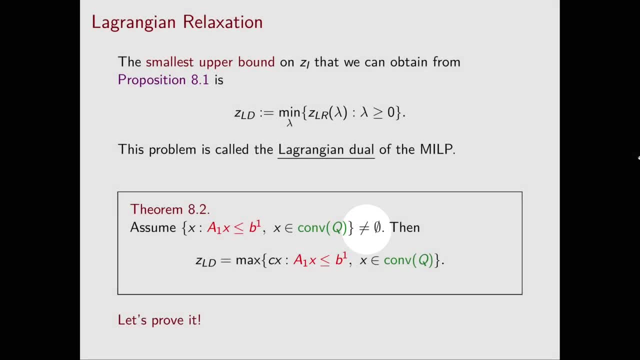 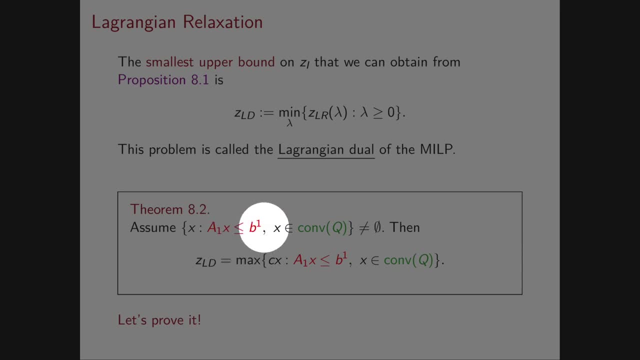 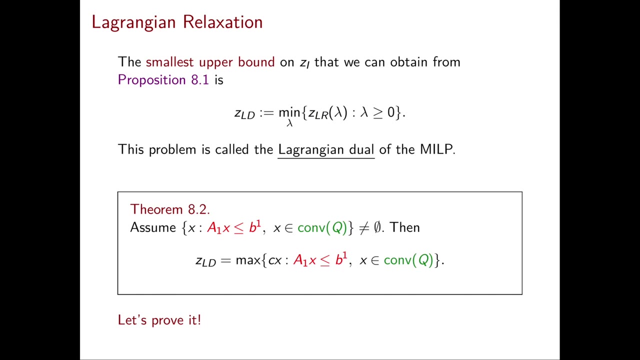 I want to briefly discuss the assumption of the theorem. Namely, we're assuming that the feasible region of this maximization problem, this set over here, is non-empty, And we saw in the proof that we in fact used this assumption. A natural question, then. 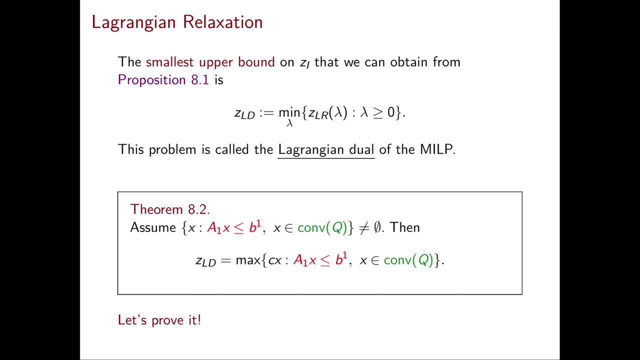 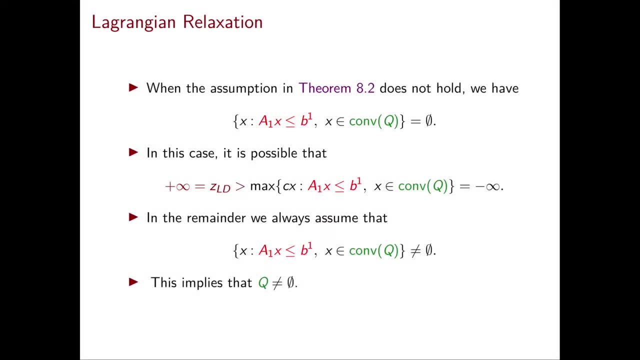 is: do we really need this assumption for the theorem to hold? And the answer, of course, is yes. In fact, you can easily construct examples where this set is empty and where not only ZLD is different from the maximization problem over such a set. 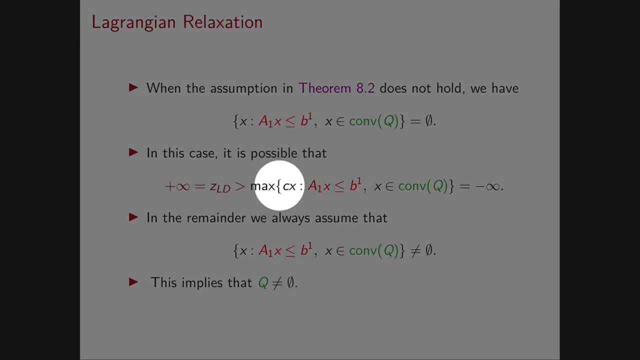 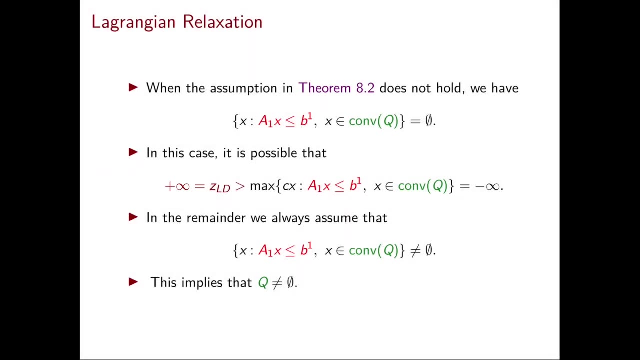 But you can actually construct examples where the max is, well, of course, minus infinity, because the feasible region is empty, And, on the other hand, ZLD can be equal to plus infinity. In particular, in the remainder of our discussion, we will always assume that this set is non-empty. 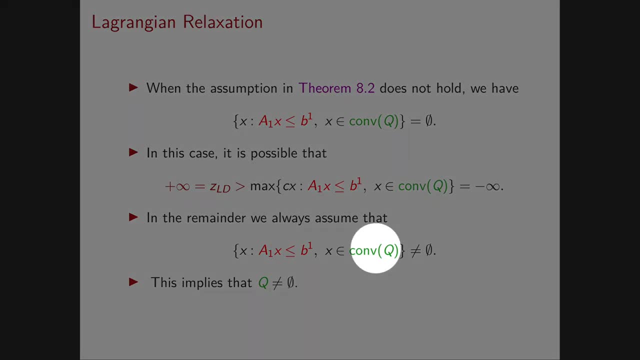 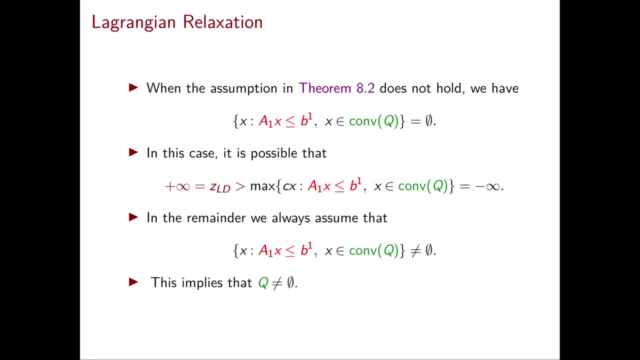 so that the theorem holds. In particular, this implies that the convex hull of Q is non-empty and therefore that Q is non-empty as well. Finally, note that this assumption is, in a sense, not a big deal. The reason is that if this set is actually empty, 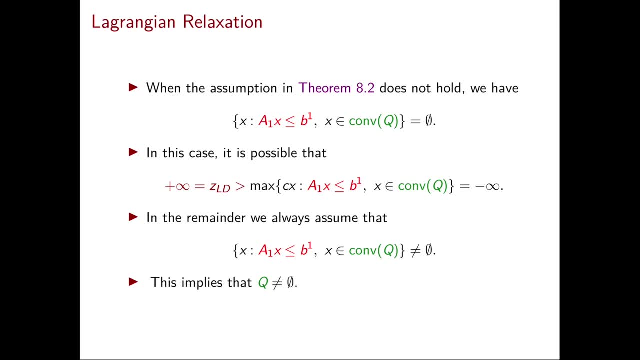 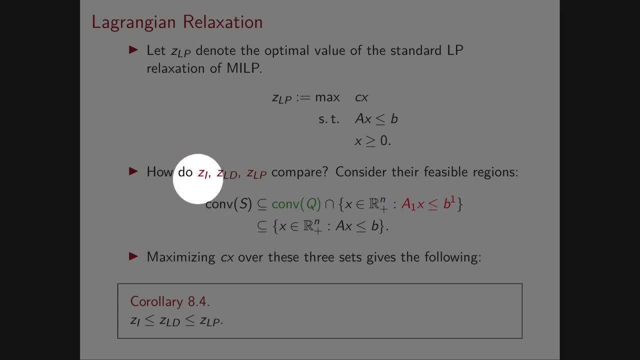 then so was the original feasible region of your problem. In this slide, I want to discuss the relationship between our true optimal value of our integer linear programming problem, our Lagrangian dual bound, and the bound obtained from the standard linear relaxation that we denote by ZLP. 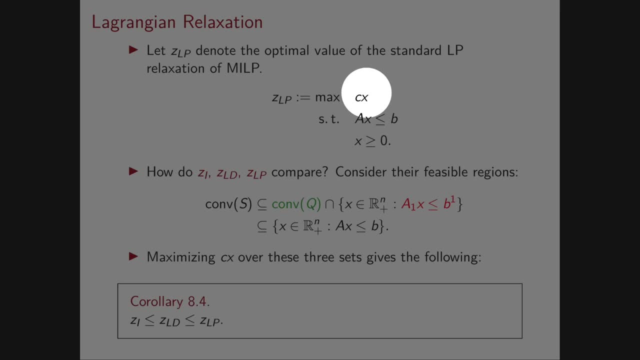 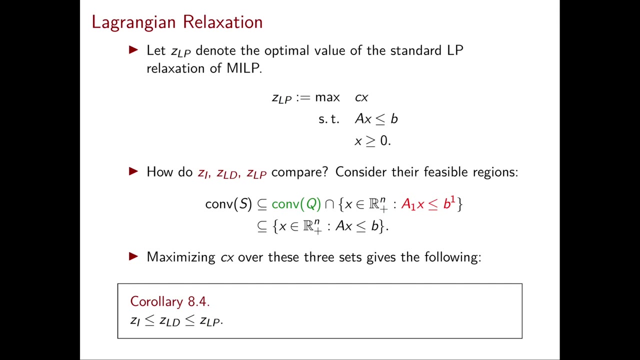 So formally, ZLP is the max of CX over the points that satisfy AX less than or equal to B and X greater than or equal to 0. So like our original problem, but we just drop integrality constraints. We know very well that both ZLD. 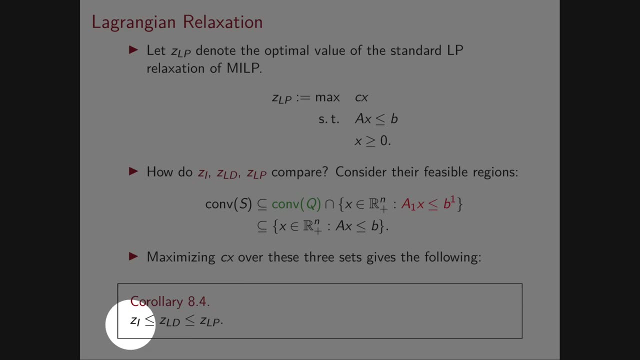 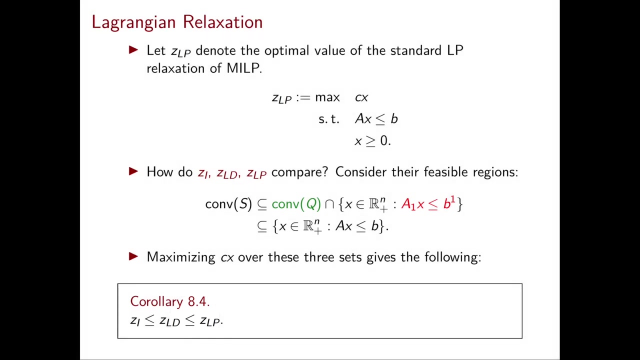 and ZLP are upper bounds on ZI. However, it is simple to see that ZLD is always less than or equal to ZLP. To prove these inequalities, we can just compare the feasible region of the three optimization problems written as linear programming problems. 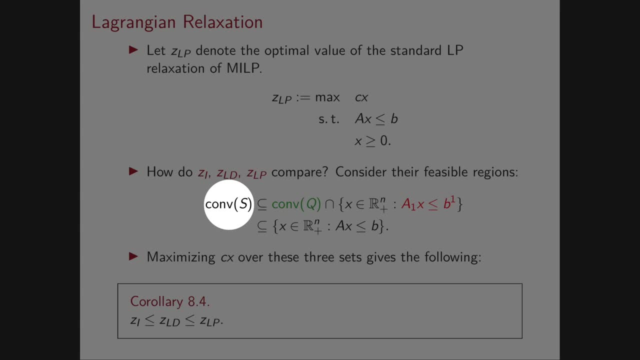 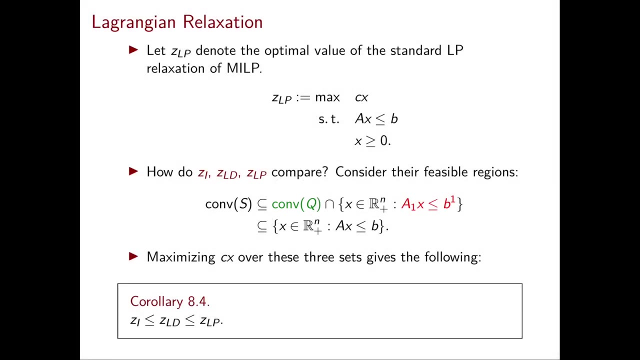 So for ZI, the feasible region is the convex hull of our original mixed integer linear set, convex For the Lagrangian dual bound. due to the theorem we've just seen, the feasible region is conf Q intersected with the set of non-negative X. 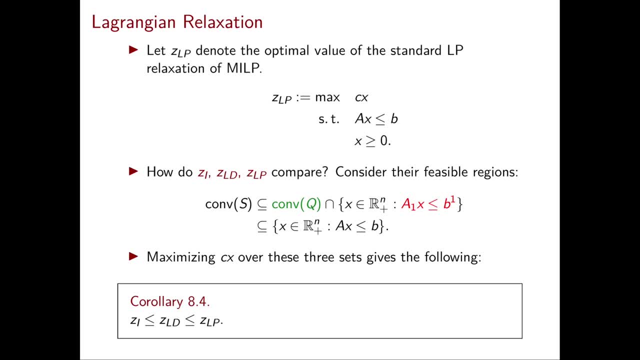 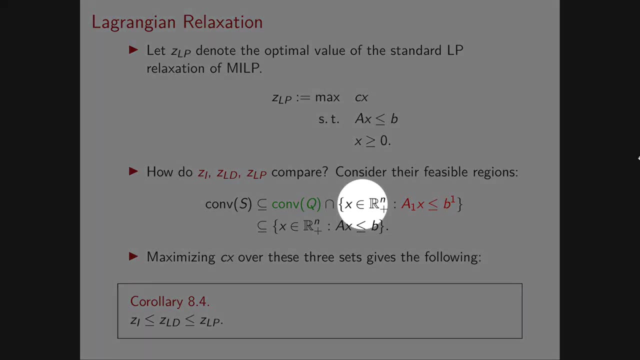 that satisfy the red system. Finally, for the LP relaxation, as we have just written, the feasible region is the non-negative vectors that satisfy AX, less than or equal to B. Now, clearly, S is contained in Q. it satisfies non-negativity, it satisfies the red inequalities. 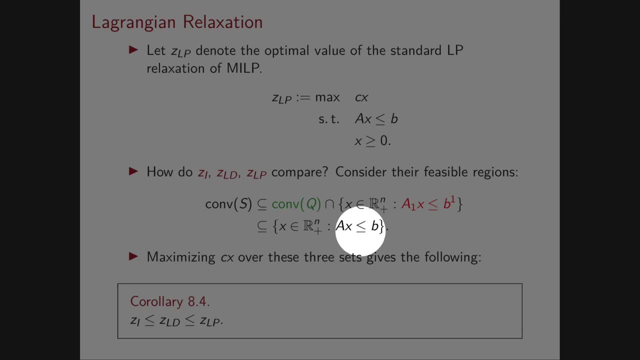 and it satisfies also the remaining green inequalities. Therefore, S is contained in this intersection and in this set, and since both sets are convex, they also contain convex, So it's clear that convex is contained in both these sets. On the other hand, 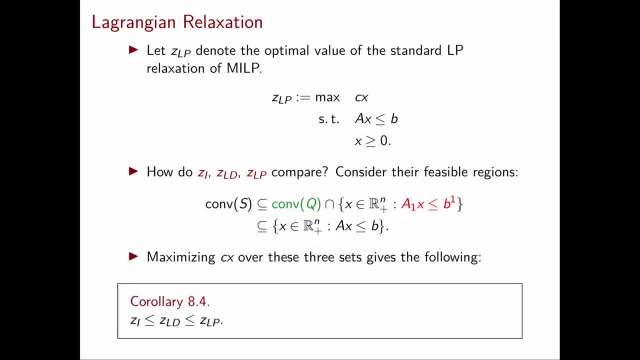 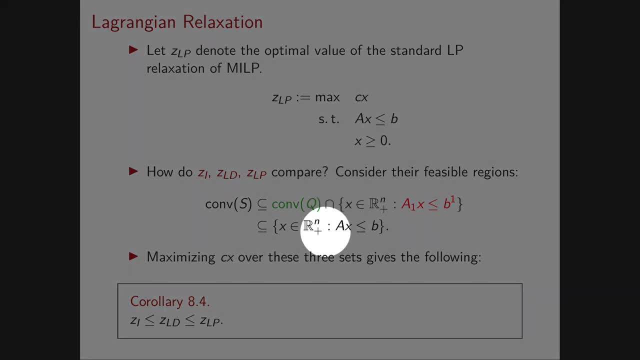 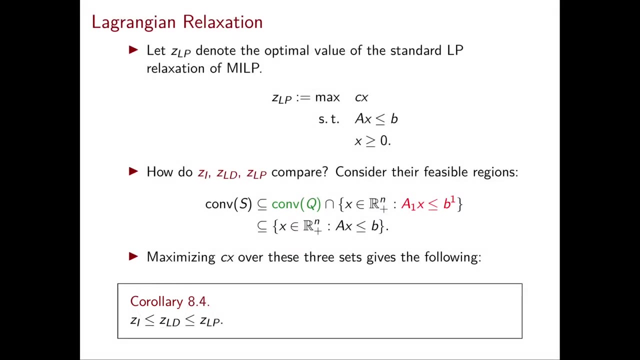 how do these two sets on the right hand compare? Clearly, conf Q satisfies all the green inequalities. Therefore this intersection is contained in the feasible region of the LP relaxation. So this simple comparison allows us to actually prove corollary 8.4.. 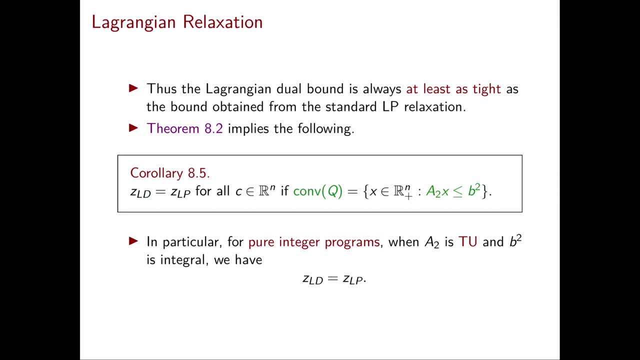 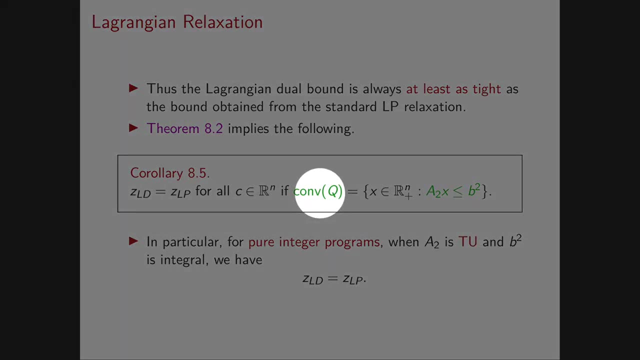 This corollary tells us, in other words, that the Lagrangian dual bound is always at least as good as the upper bound obtained from the standard LP relaxation. Of course, in some cases these two bounds can coincide, For example whenever the convex hull of Q. 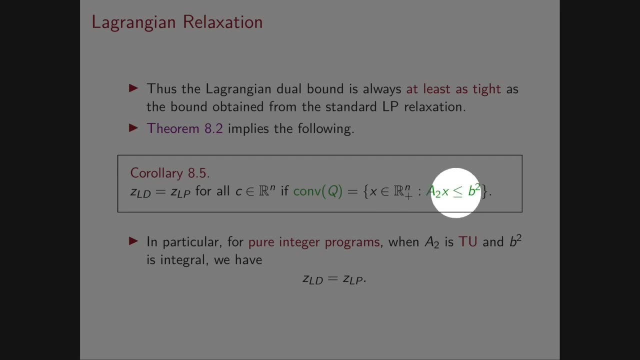 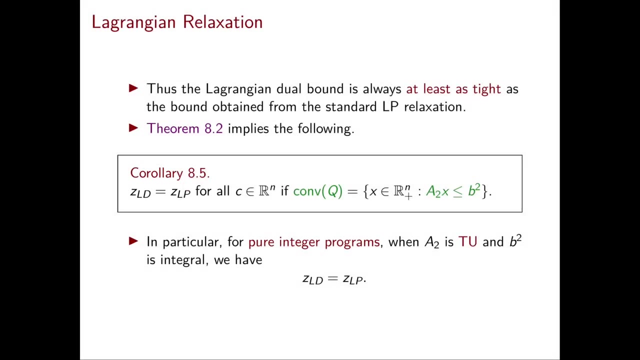 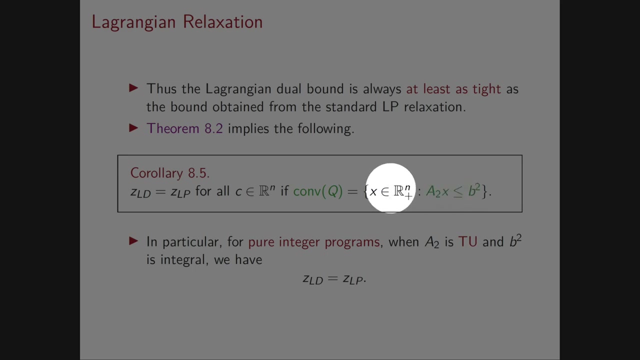 is exactly defined by the green: inequality and non-negativity, then we obtain that the Lagrangian dual bound is equal to the linear programming bound. Recall that Q is defined exactly as the set of mixed integer points that satisfy these conditions. Therefore, asking for this condition, 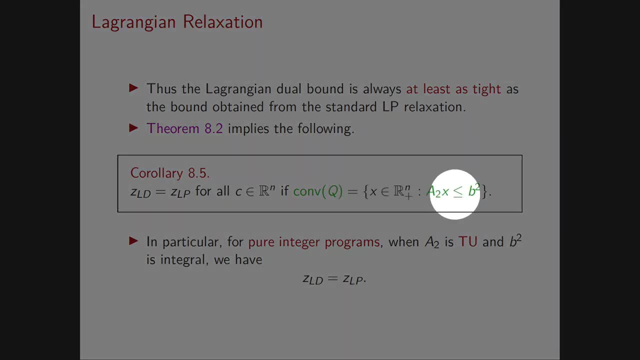 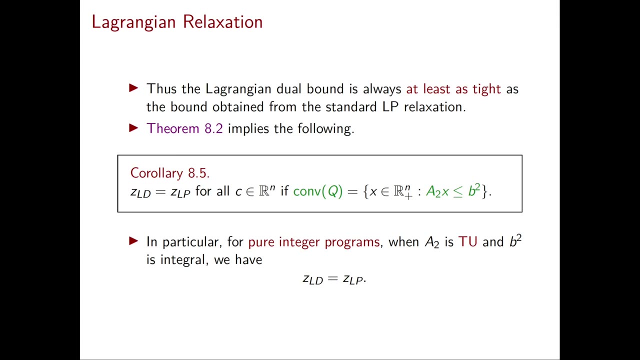 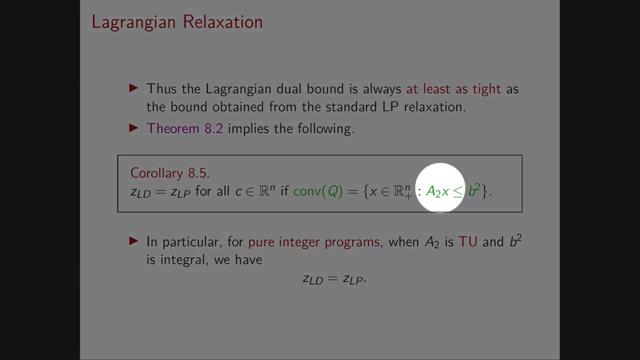 is equivalent to asking that this system gives you a perfect formulation of the set Q In chapter 4,. we have, of course, seen several examples of perfect formulations And, for example, if all the variables are required to be integral, if a2 is totally unimodular. 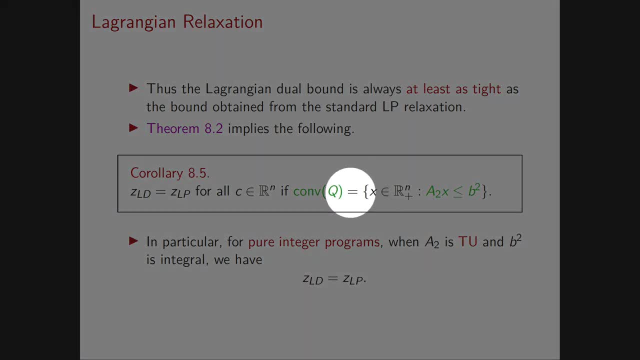 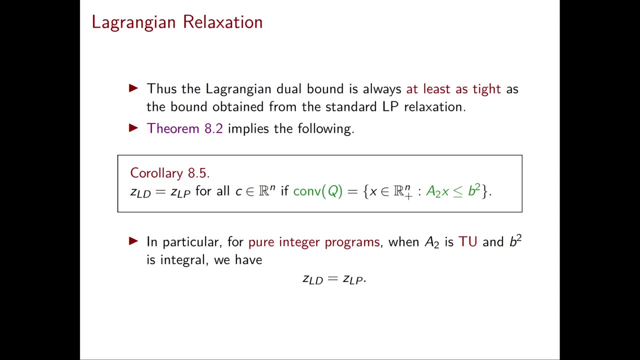 and b2 is integral, then our sufficient condition is satisfied and therefore we obtain that the Lagrangian dual bound is equal to the linear programming bound. In the next few slides we're going to look at a specific example of a Lagrangian relaxation. 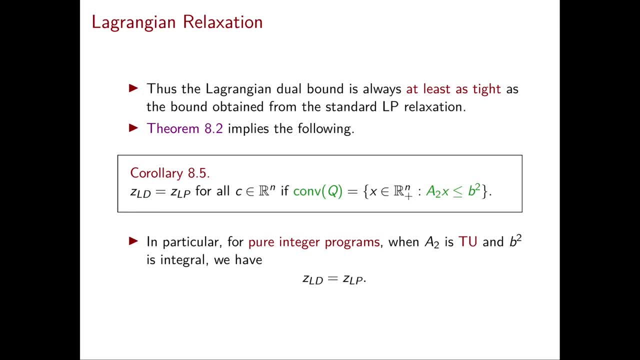 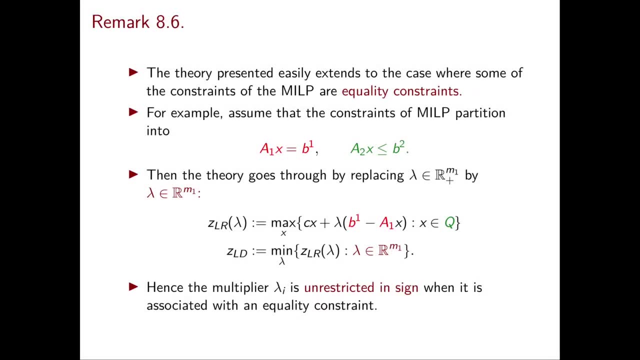 applied to the traveling salesman problem And for that example, we're going to need to apply the theory that we developed in a slightly different form. Namely, some of the constraints of the mixed integer linear programming problem will be equality constraints. Therefore, let's see: 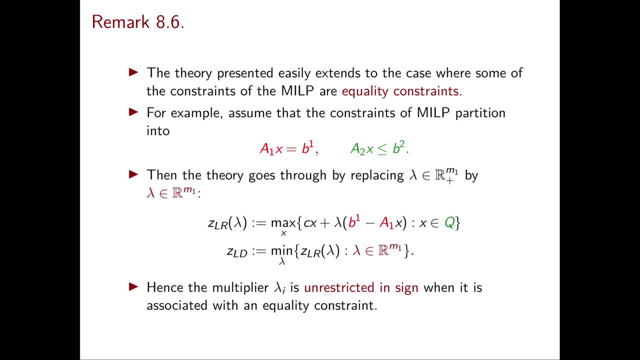 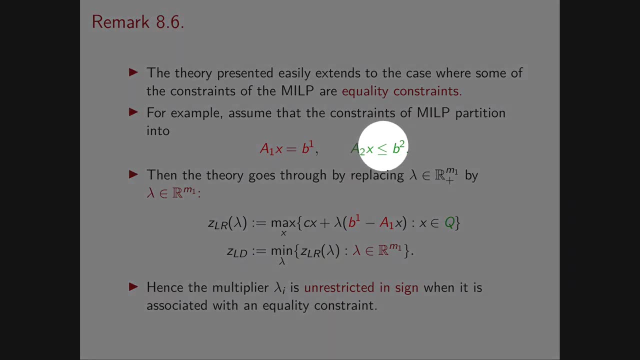 in general, how the theory that we developed changes if we have some equality constraints in our original formulation. For example, think about a setting where we have that our red constraints are all at equality, while the green constraints are, as before, in the form less than or equal to. 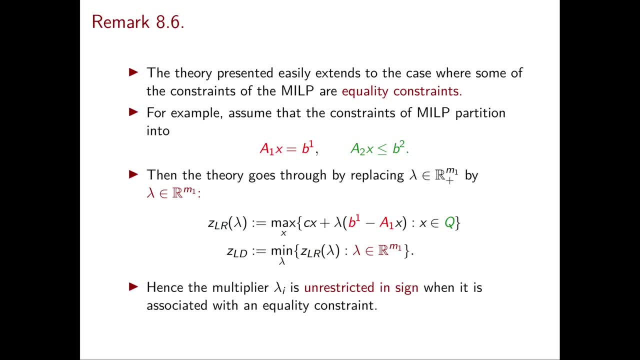 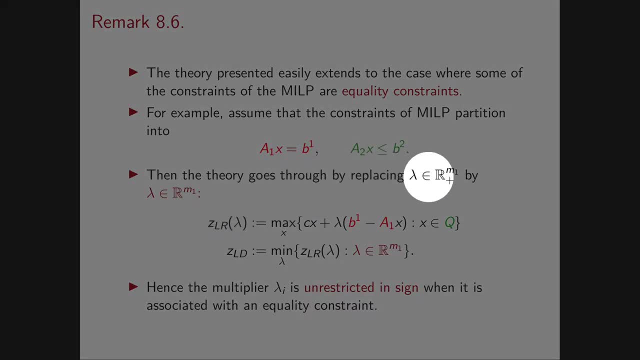 Then we define the set Q in the same exact way, and this makes sense, because the inequalities that are green didn't change at all. On the other hand, the multiplier's lambda will change, because they weren't required to be non-negative, and now instead they will be just free. 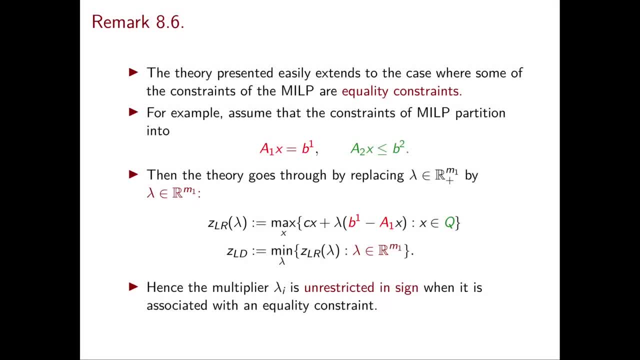 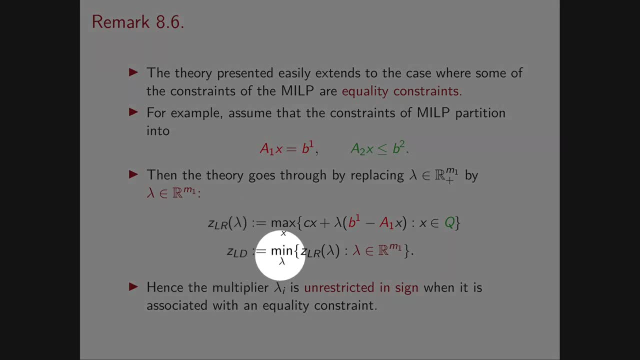 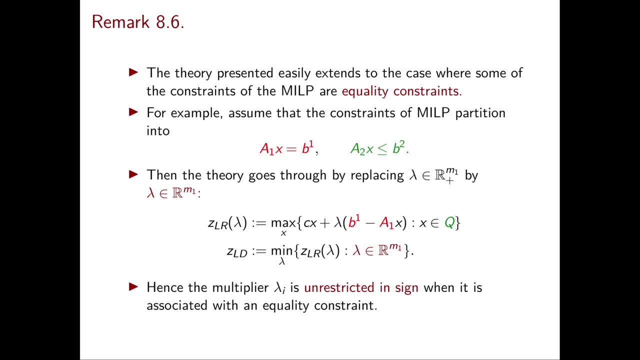 Therefore, the Lagrangian relaxation will be defined for every lambda and the Lagrangian dual will be the minimum over all lambda in RM1, without the constraints that lambda has to be greater than or equal to zero. More generally, you could of course have 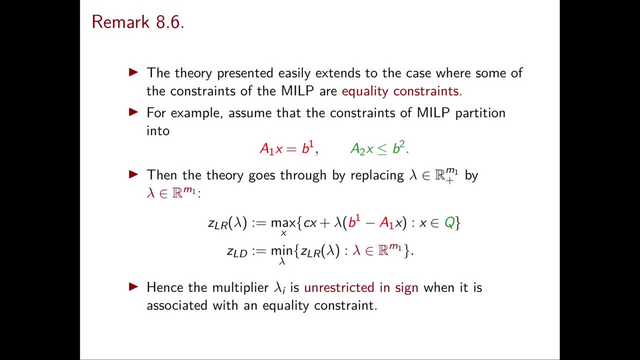 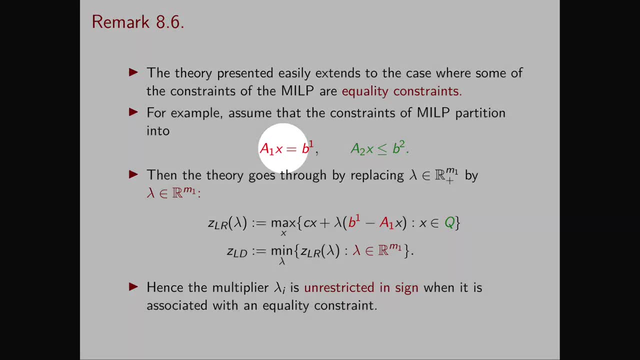 some inequalities of the form less than or equal to in here and some equality constraints. In this setting, as you can imagine, you will have that the lambdas corresponding to the inequality constraints will have to be greater than or equal to zero and the ones corresponding 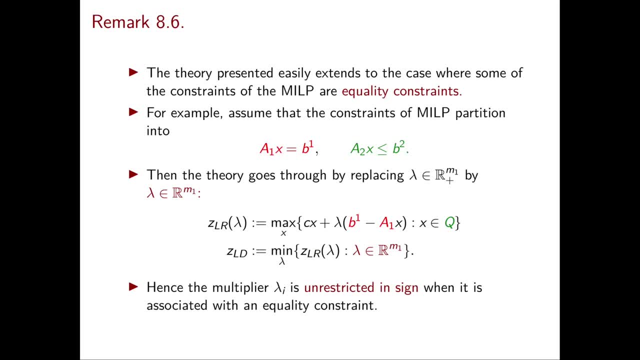 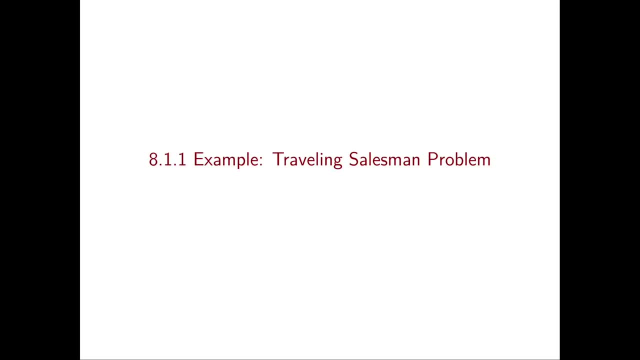 to the equality constraints will be instead free. Now that we've clarified this kind of different forms of Lagrangian duality, let's look at our example. So let's focus on the traveling-seismen problem In particular. we want to discuss. 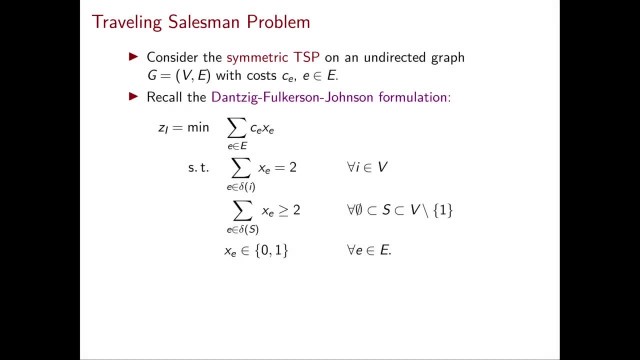 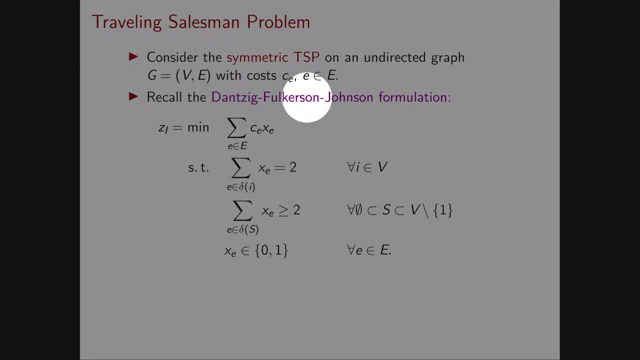 the symmetric TSP problem on an undirected graph with cos CE, as we have already discussed in chapter 2.. We saw the Danzig-Fulkerson-Johnson formulation Recall that we have degree constraints on every node and we have subtour elimination constraints. 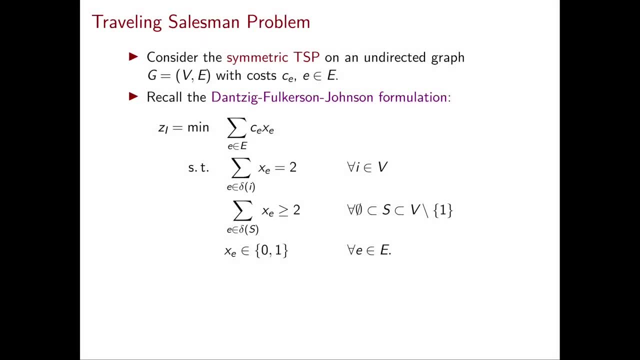 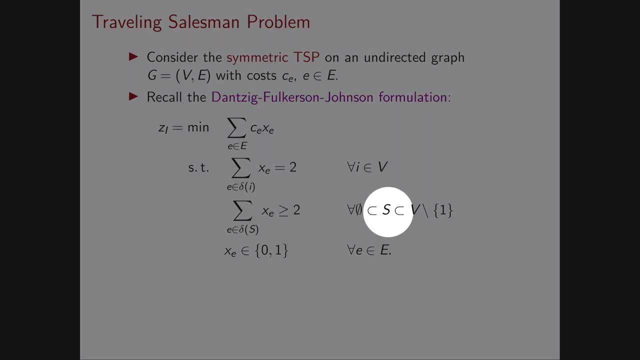 However, note that there is a subtle difference with respect to the Danzig-Fulkerson-Johnson formulation that we have already seen. So, if you remember, in the original formulation that we have seen here, we add every subset of V. that was non-empty. 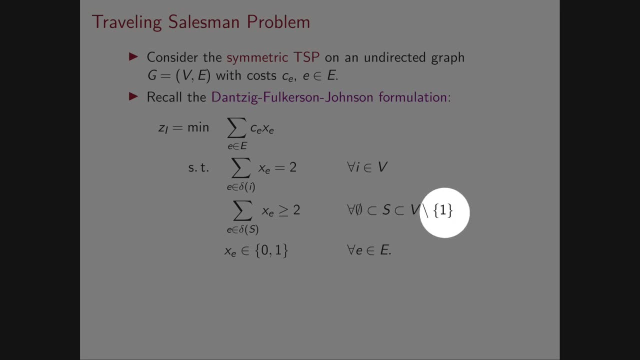 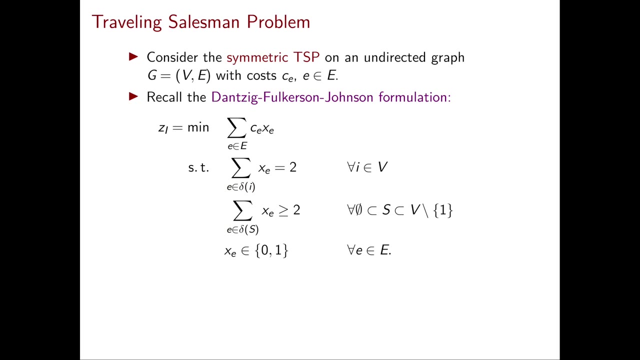 and not equal to V. So essentially, we didn't have this set minus 1.. So the question is: why can we actually write down here a minus 1 without changing the formulation? Well, the reason is very simple. In fact, for every set S, 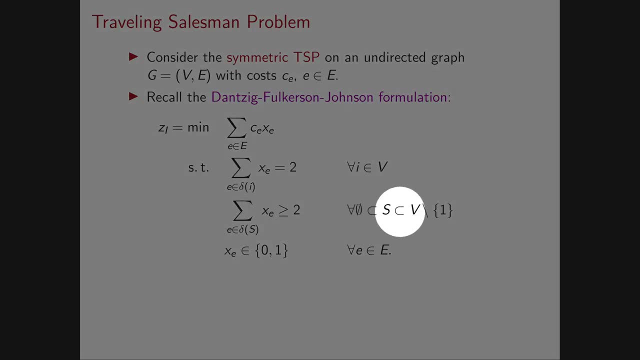 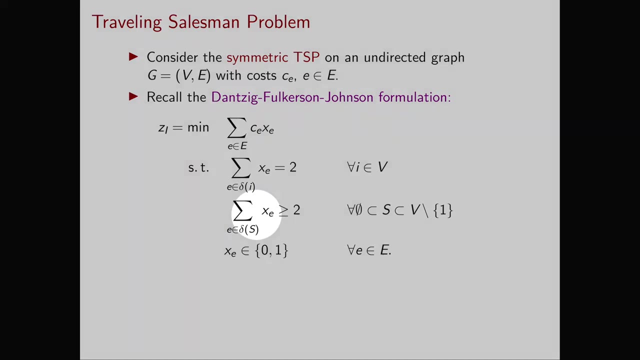 that is contained in the empty set and contained in V. if we take the inequality corresponding to S and the inequality corresponding to V minus S, you obtain the same exact inequality. So essentially, among these two, for every set S, you can keep only 1. 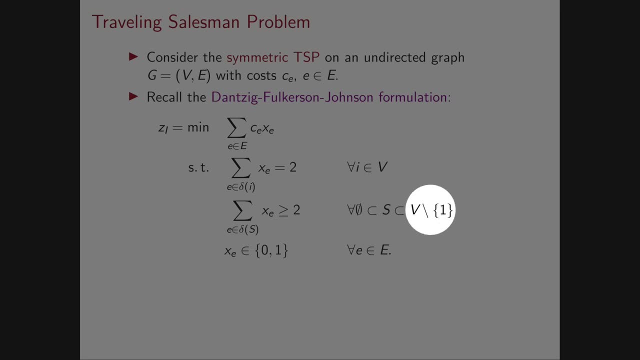 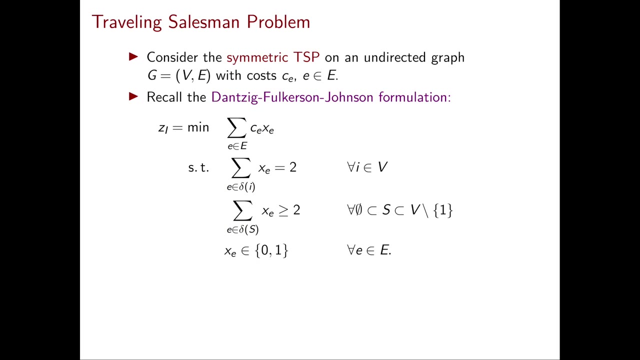 and you can always throw away the one containing node 1.. So, essentially, this formulation is obtained from the original dancing-Fulkerson-Johnson formulation that we've already seen, by just throwing away, for each pair of these identical inequalities, just the one containing node 1.. 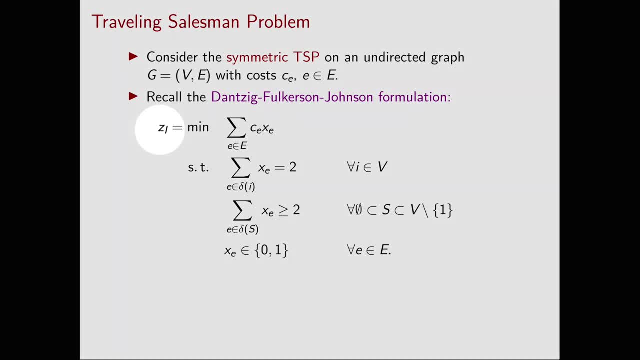 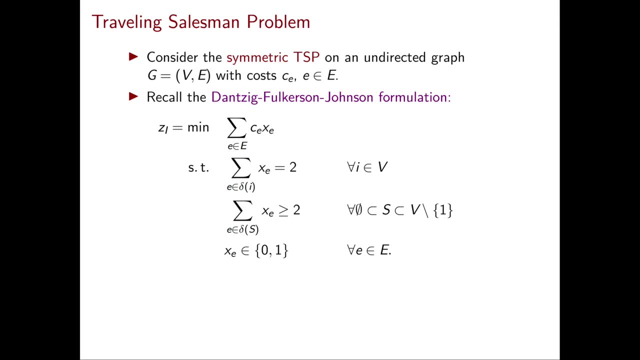 We're going to denote the optimal value of this problem by Zi, as we're doing in this chapter, Before constructing a Lagrangian relaxation of this problem. I want to massage a little bit this formulation. So the first thing I want to do is rewrite: 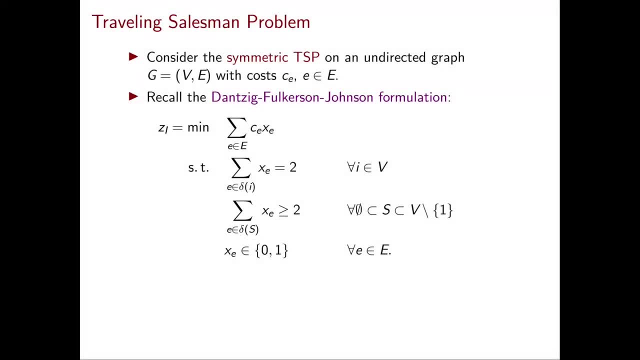 the subtour elimination constraints in a slightly different way. The reason I can do that is because I have equalities that I can always use in order to essentially tilt my inequalities, so that their intersection with a fine hull of the polyhedron remains the same. 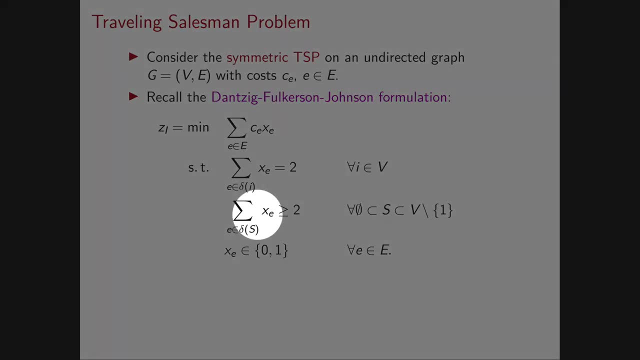 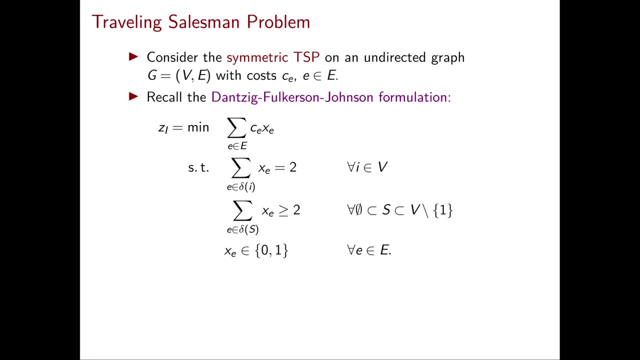 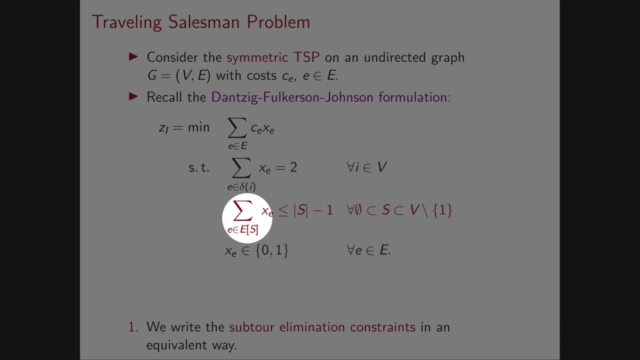 In particular, while the current subtour elimination constraints tell us that you must have, for every set of nodes, at least two edges leaving the set, we're going to write them in this equivalent form. In this form, we're looking at the sum of the axes. 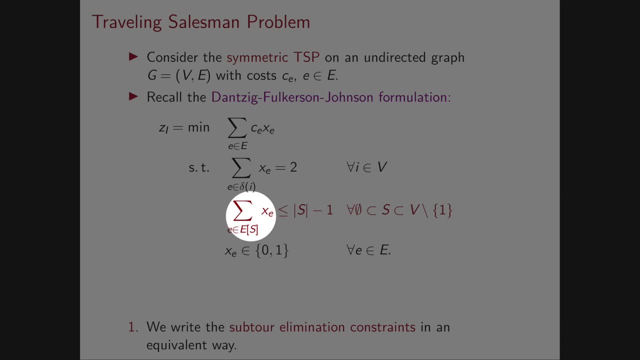 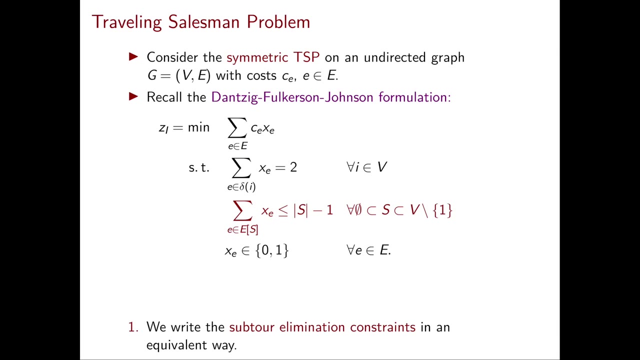 for every E fully contained in the set S, and we're asking that this sum is, at most, the cardinality of S-1.. It's a very good exercise to show that these inequalities are equivalent to the previous ones and, of course, in order to show that 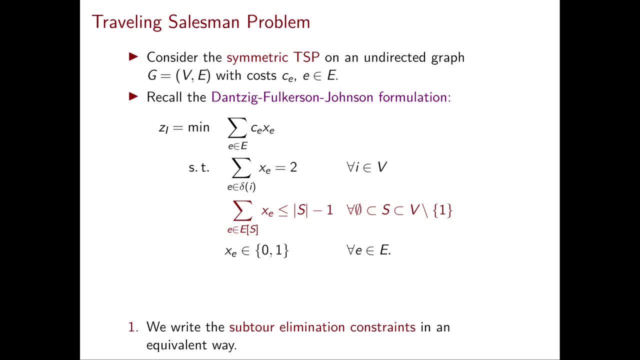 you need to use the degree constraints. The next step to this formulation is, in a sense, trivial, because we're just going to add one constraint that is redundant. In fact, it's already implied by all our equations. In fact, if you sum the degree constraints, 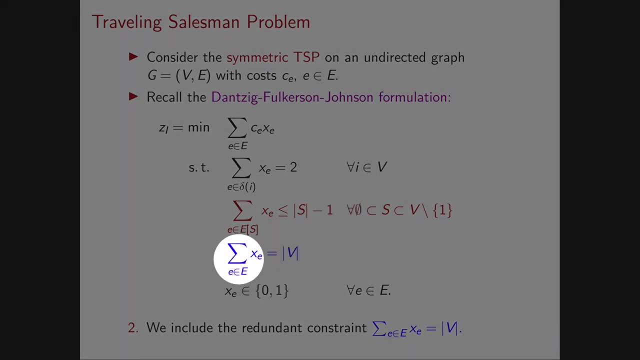 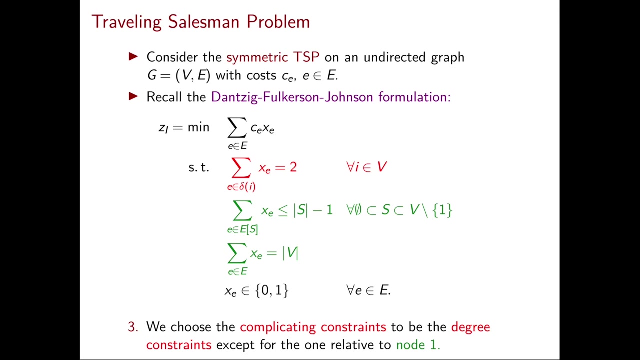 for every node, you obtain that twice the sum of all the axes is equal to twice the cardinality of V, and therefore this equation is then obtained by dividing by two such a sum. So, in order to construct the Lagrangian relaxation, now I have to choose. 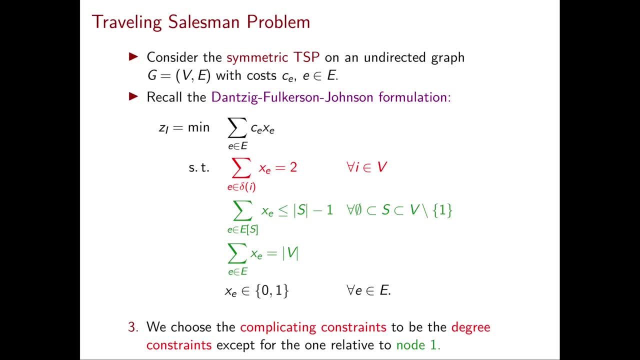 which are the complicated constraints that I want to bring in the objective in the Lagrangian relaxation, and the choice that we make at this point is to pick as the complicated constraints all the degree constraints except for the one corresponding to the node one. For some reason, 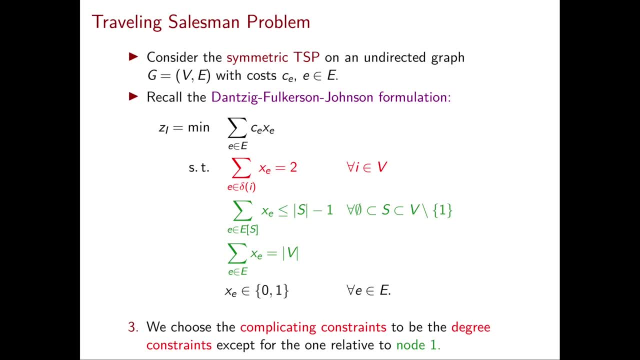 I want to keep this very specific degree constraints among my constraints. So so far all the problems. as it's written still gives me z? i. now let's write down the Lagrangian relaxation which will give me instead z l? r. Here it is. 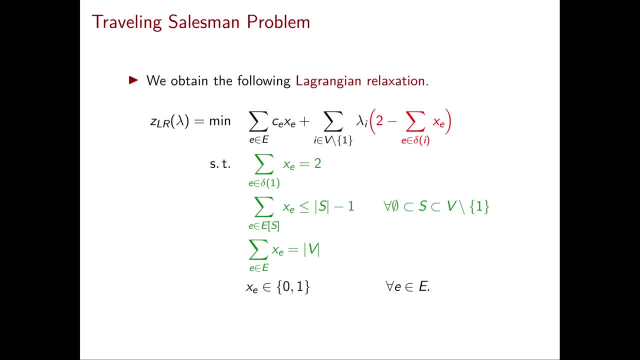 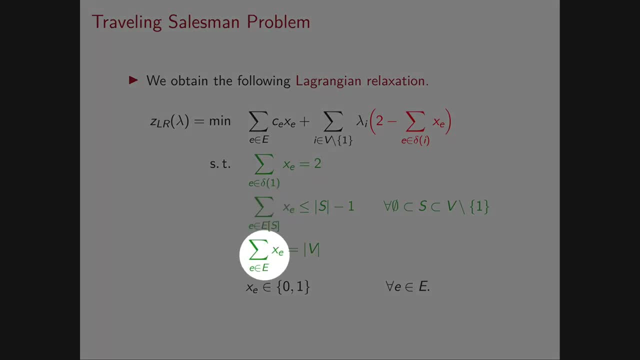 as promised, I kept among my constraints the degree constraint only corresponding to node one. I still have all my subtour elimination constraints and I have the redundant equality that I have added. Then I have brought in the objective, the Lagrangian relaxation term corresponding to all. 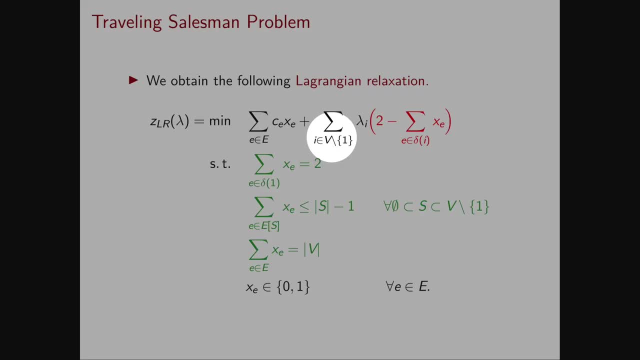 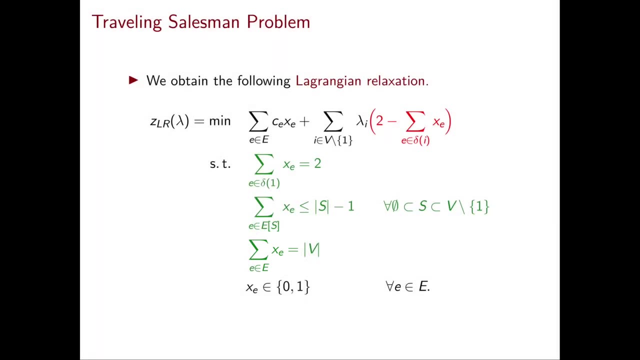 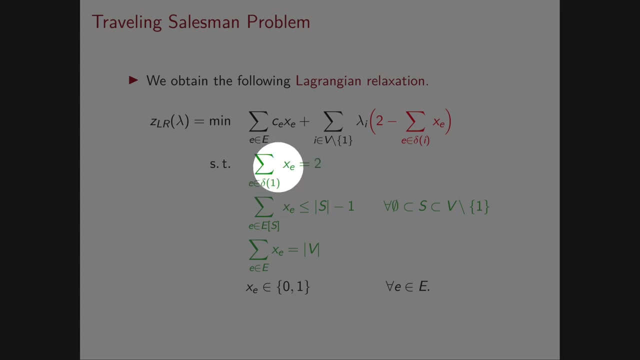 the degree constraints for every node except for node one. A key observation is that at this point the inequality that was redundant before is no longer redundant for the current Lagrangian relaxation, because I don't have all the other equalities that used to imply such 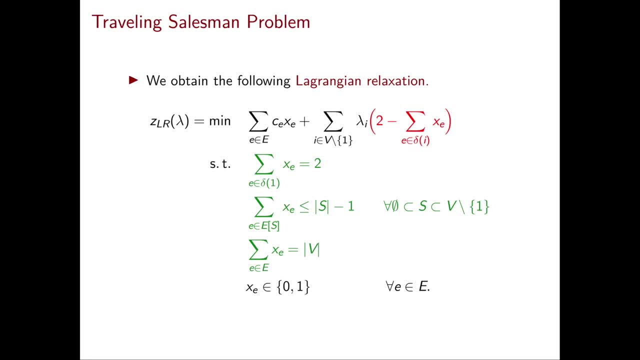 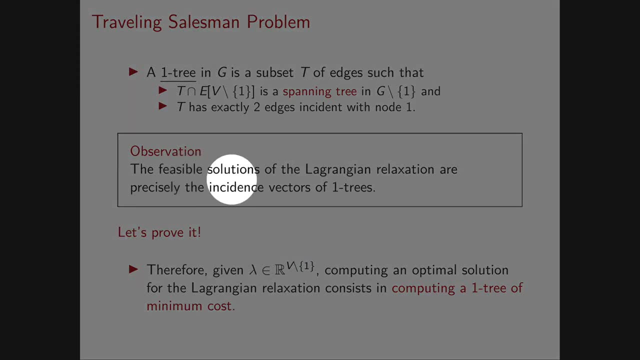 constraint. Now let's look at the Lagrangian relaxation as an interesting combinatorial object. In fact, in this observation, we are going to show that the feasible solutions of the Lagrangian relaxation are precisely the incidence vectors of one trees. What are? 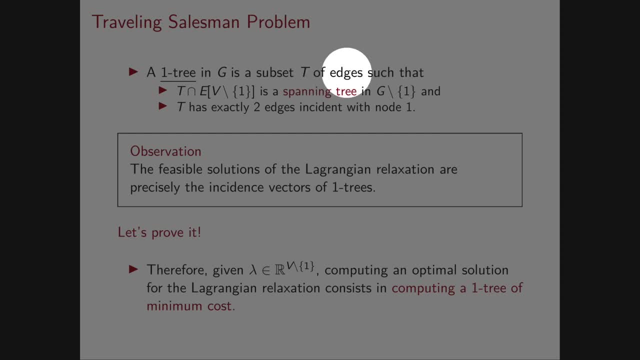 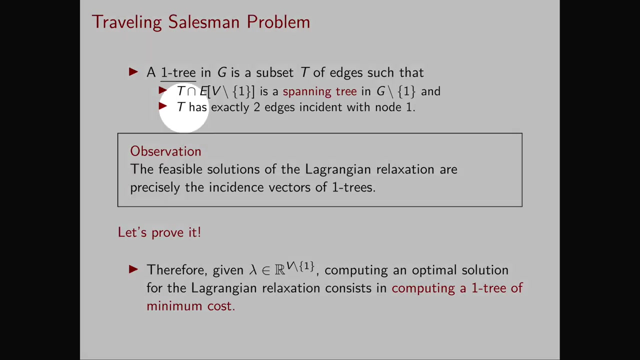 one trees. Let's see their definition. A one tree in our graph is a subset of edges such that first, an edge forms a spanning tree in the graph obtained from G by removing the node one, And secondly, T must have exactly two edges. incident. 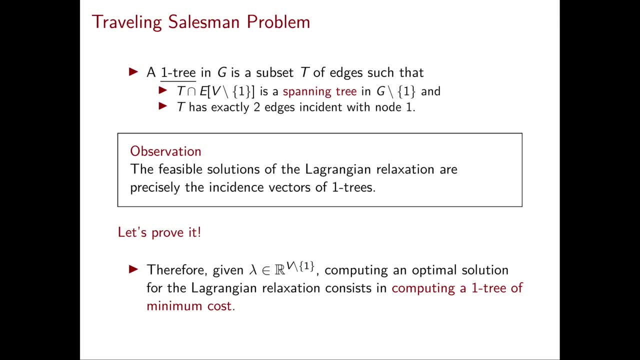 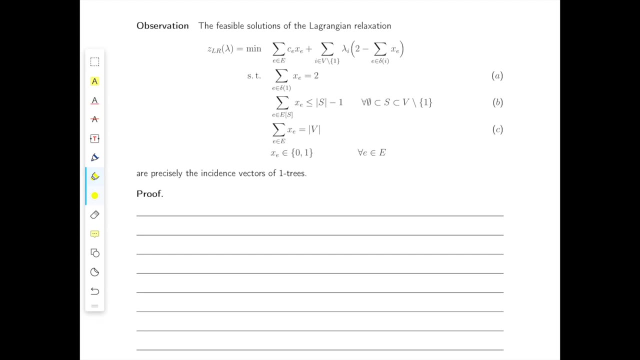 with node one. Note that in this definition, we are considering completely separately the edges that are not incident with node one and those that are incident with node one. Now let's prove this observation, The idea to prove that one tree treats separately the edges that are. 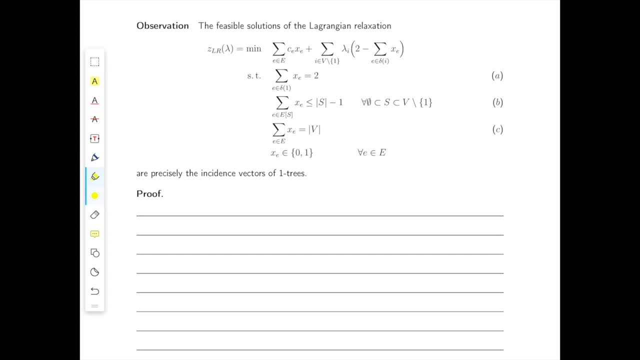 incident to node one and those that are not. So we should obtain the same thing in our inequalities. Therefore, we want to partition the constraints of the system in such a way that one of the two partitions only contains variables corresponding to edges incident to node one. 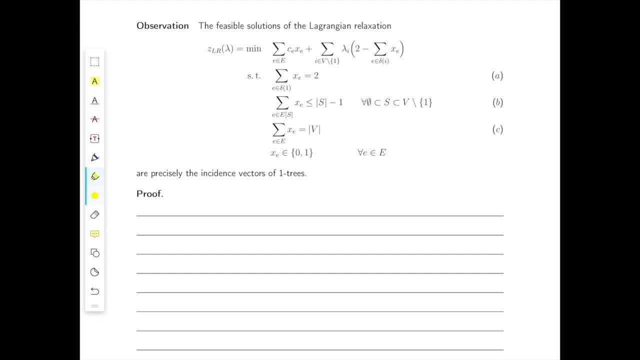 and the other partition only contains all the other variables. therefore, we need to add currently what we have. Well, the first constraint definitely deals only with variables incident to node one. Our sub-tour elimination constraints, on the other end, only deal with variables that are not. 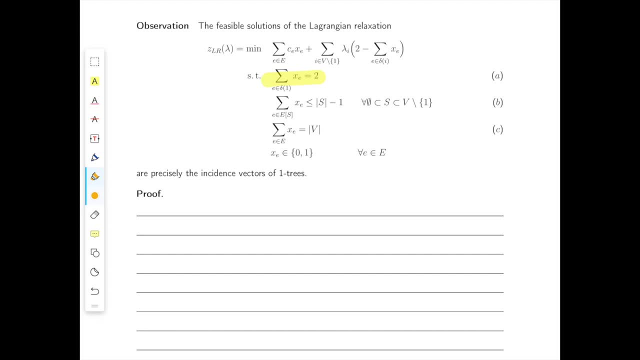 incident to node one. That's because we are only considering subsets of nodes that don't contain node one, So let's highlight this in a different color. Finally, the last constraint that we have contains all variables that we need to change in this formulation. and how are we going? 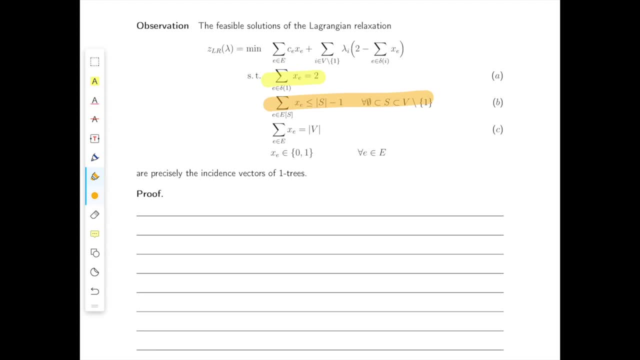 to do that? Well, we're going to remove from it the inequalities A, so the ones highlighted in yellow here, and obtain in such a way an equation containing only variables of edges that are not incident to node one. Let's do it In our system. 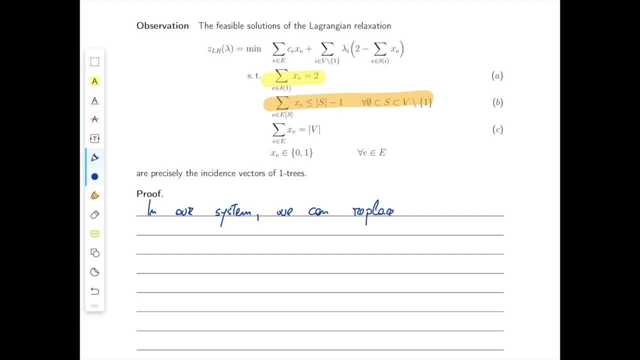 we can replace constraints C with the one obtained subtracting A from C, which is sum for E in capital, E minus delta of one of X, E equal to cardinality of V minus two, And let's call this equation C prime. We have achieved now 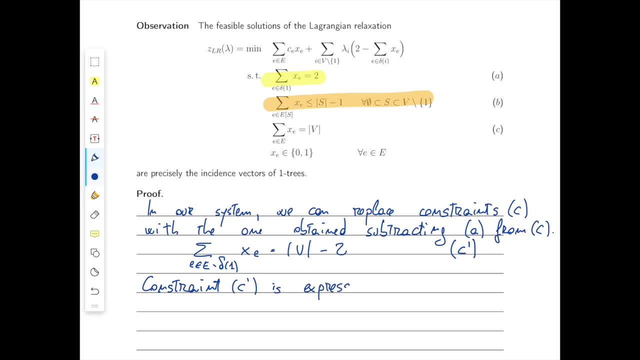 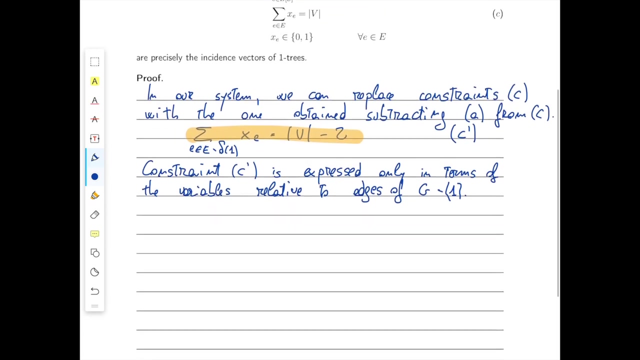 our goal, because constraint C prime is expressed only in terms of the variables relative to edges of G minus one. So essentially I can highlight it in orange. So now we can write our feasible set as a product. Let's do that, So we have. 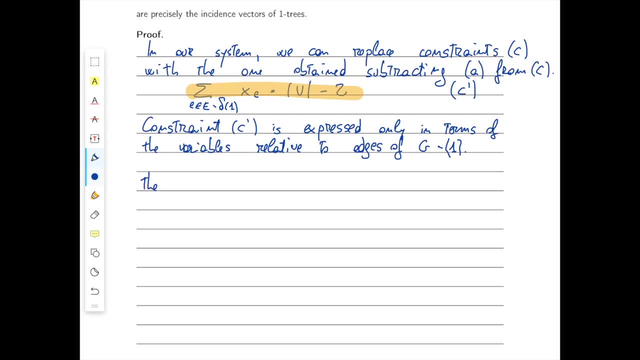 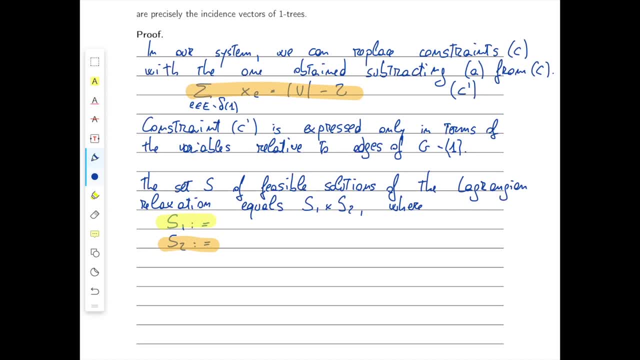 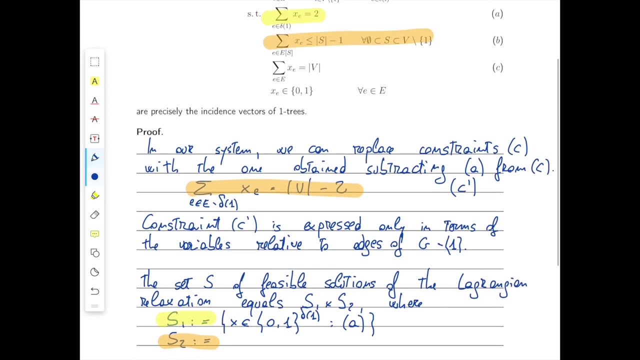 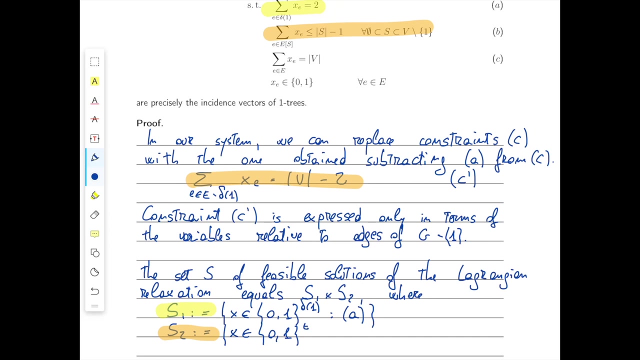 will be our yellow set. So S1 is the set of binary points in dimension delta of one that satisfy only A, which, if we go back, is our only equality, while S2 is equal to the set of X's in 0,, 1,, 2,, d, e, minus delta of 1. such 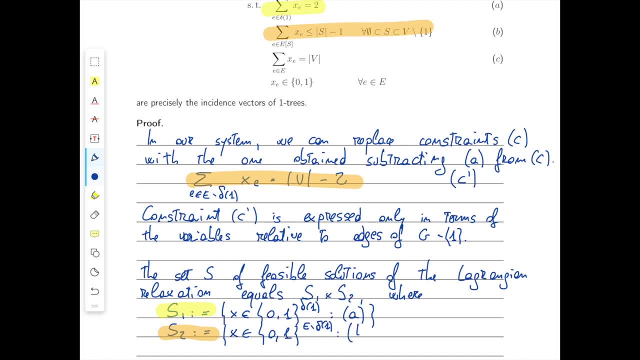 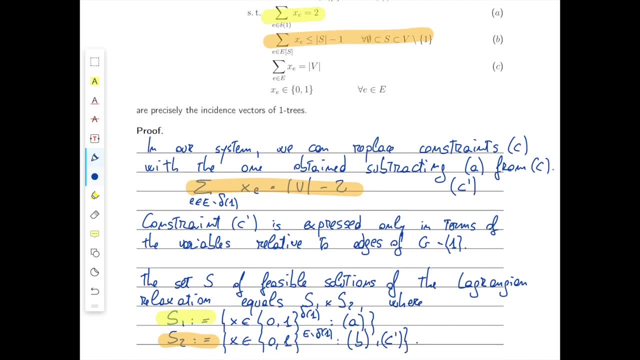 that the orange inequalities, which are b and c prime. at this point we can analyze these two sets separately, so let's look at a yellow one. so these are all the binary points that satisfy only a, this yellow equation, and so it is exactly the set of incidence factors, of subsets of delta, of. 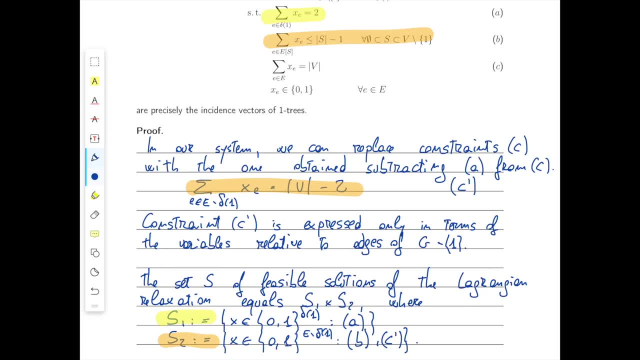 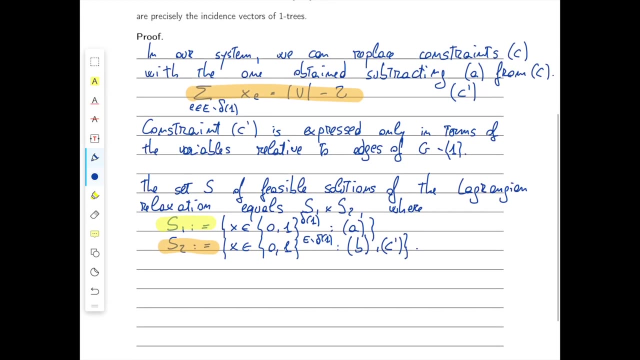 one of cardinality two. on the other hand, what is S2? the set? S2 satisfies the orange equation c, prime and all the inequalities b, and we have seen this system before because it describes the spanning trees in G minus 1. let's write it down: S1 is the set. 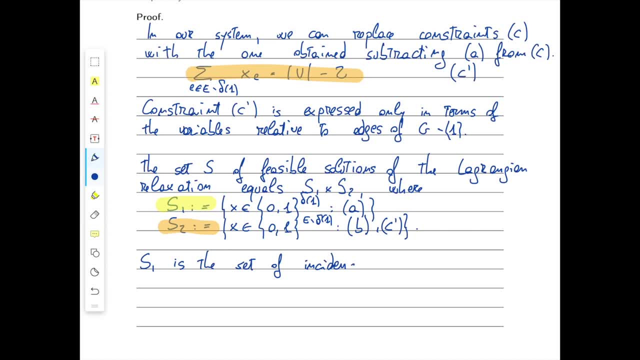 of incidents, of the incidence factors of subsets of delta1 of cardinality2, and this 2 is the set of incidence factors of spanning trees in g-1, which is exactly our definition of one tree, and so this concludes our proof. Back to the slides. 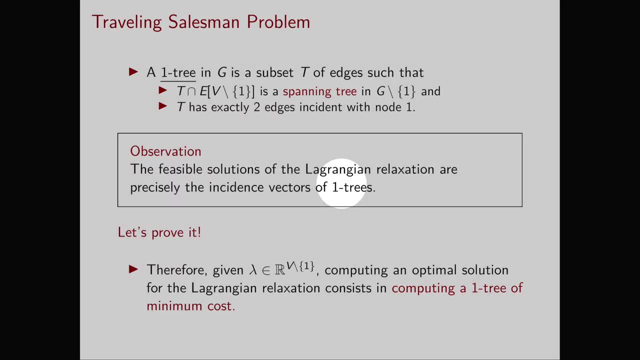 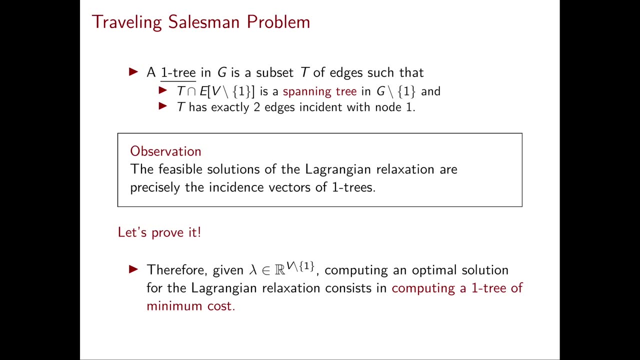 We have just shown that the feasible solutions of the Lagrangian relaxation are the incidence vectors of one tree. Therefore, for every given lambda in our Lagrangian relaxation, solving such a relaxation consists in finding a one tree of minimum cost where, once again, the cost depends on lambda. 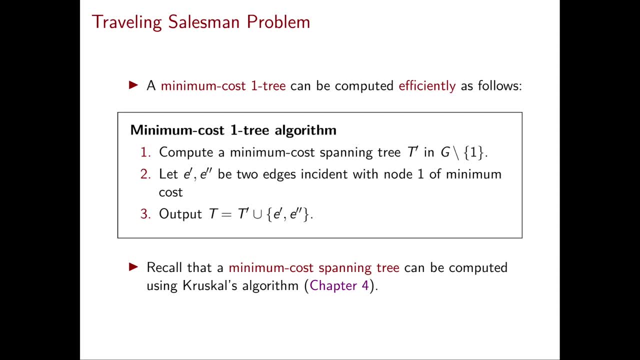 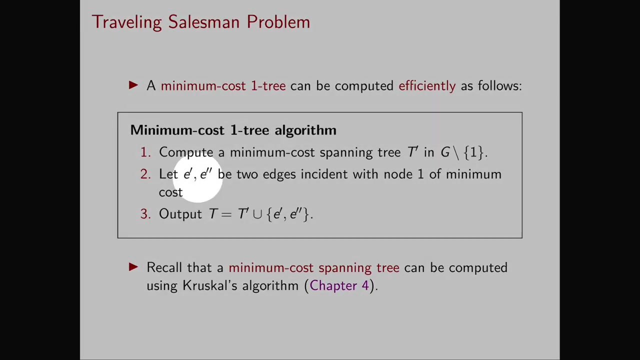 Now the definition of one trees we've seen essentially treats separately the edges incident to node 1 and the other edges. Therefore, in order to compute a minimum cost one tree, we can separately optimize these two structures. So here is our algorithm: We compute a minimum cost spanning tree t' in g-1 and then we pick the two edges e'. 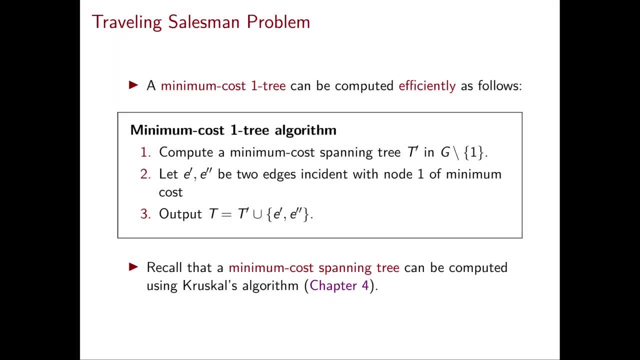 e'' incident with node 1 of minimum cost, Then our minimum cost one tree is the union of t' and e' e''. Clearly step 2 can be done in linear time. And regarding step 1. We have seen that Such a minimum cost spanning tree can be obtained, for example, with Kruskal's algorithm. 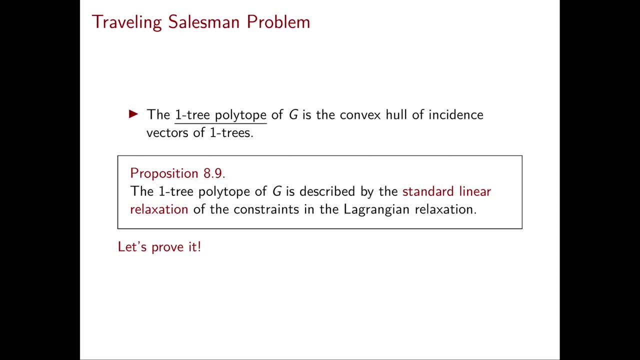 We're also in a position to fully characterize what is called the one-tree polytope, which is the convex hull of the incidence vectors of one trees. In the next proposition, we will show that the feasible region of our Lagrangian relaxation is in fact a perfect formulation. 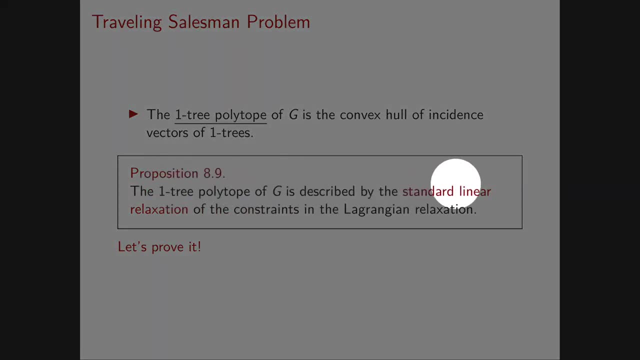 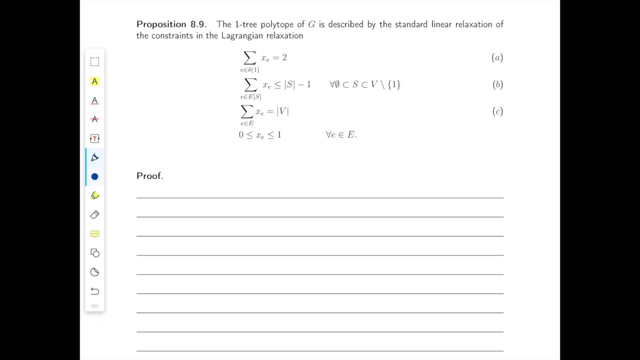 We're going to show that the one-tree polytope of G is described by the standard linear relaxation of the constraints in the Lagrangian relaxation. Let's show this In the statement. here I have explicitly written down the standard linear relaxation of the constraints in the Lagrangian relaxation. 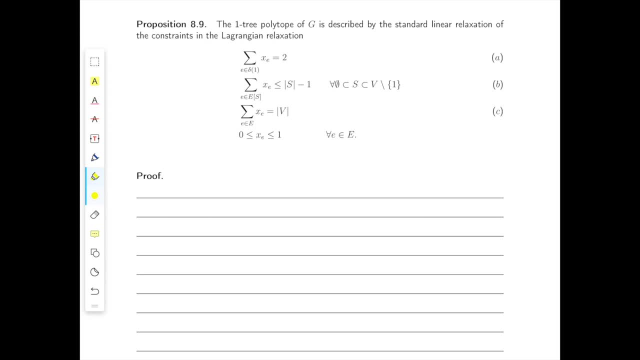 In fact, note that it's the same exact system, except for the inequalities xe between 0 and 1, which replaced the binary constraints that we had in the formulation. Well, there's not really much to do in this proof. Essentially, I'm just going to use what we've done in the observation. 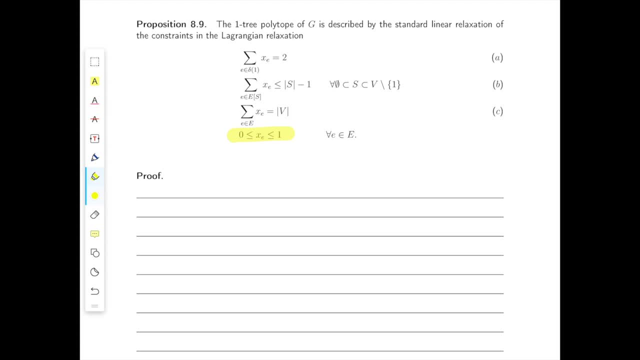 I'm going to use the theorem that we saw in chapter four that characterizes the spanning one-tree polytope, and I will leave the rest as an exercise, The proof, like the one, of the observation we want to partition our constraints into. 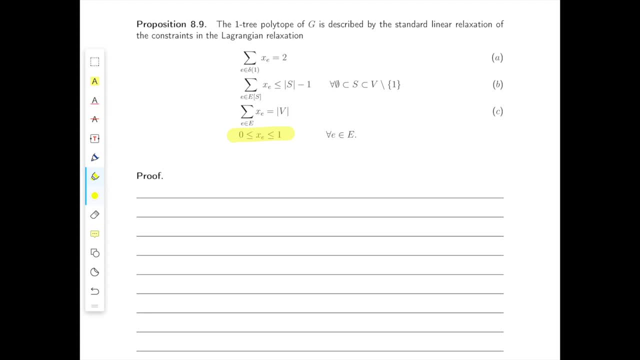 two sets. One set will contain only the variables corresponding to edges incident to node one, and the other partition contains all the other variables. So let P be the polytope, So let P be the polytope. So let P be the polytope. 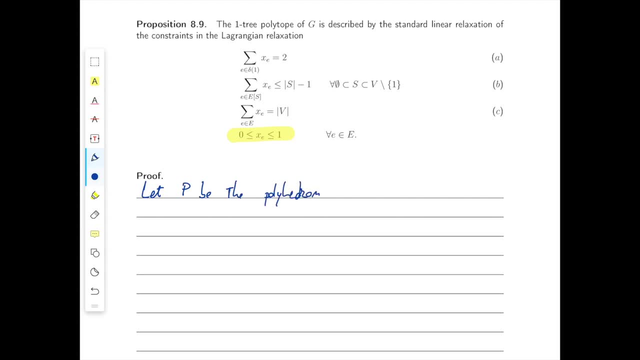 So let V be the polyhedron described by the standard linear relaxation of the constraints in the Lagrangian relaxation. It follows from the proof of the observation that P can be written as a product of polyhedra: P1 times P2, where 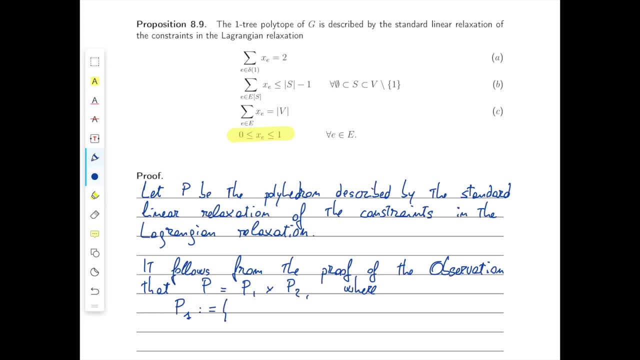 P1 is the set of vectors with components corresponding to edges in delta of 1 and in the interval 0, 1 that satisfy only constraint A. and P2 is the set of X in again 0, 1 in the space of E minus delta of 1, such that B and C prime. 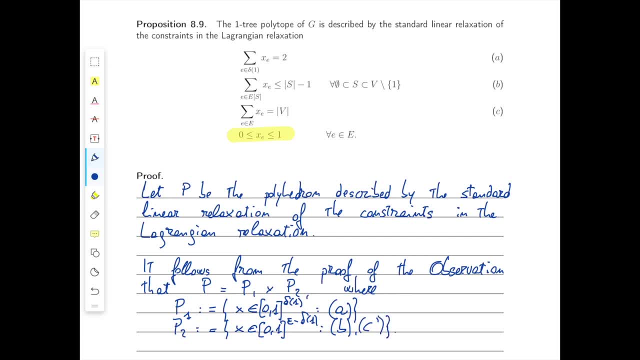 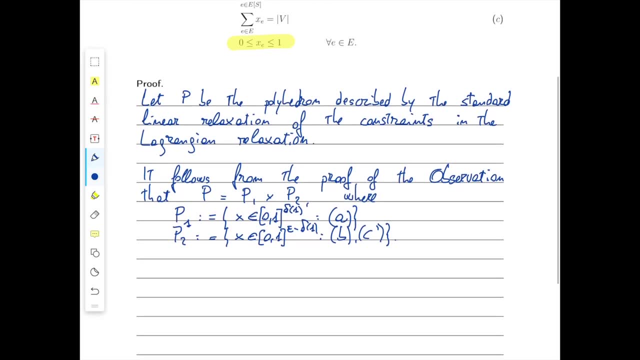 So this is exactly the same thing we've done in the observation, but this is the corresponding linear relaxation of the sets S1 and S2 that we saw there, And now we just have to study separately P1 and P2.. It is easy to see that. 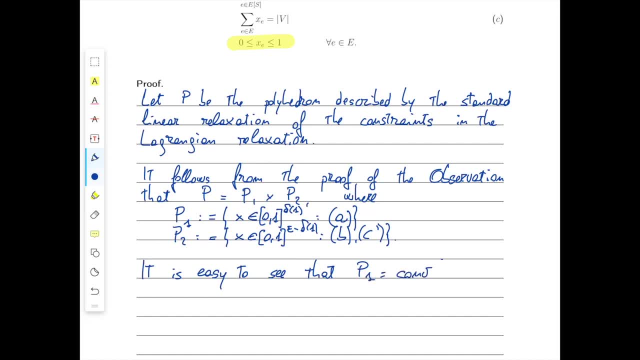 P1 is the convex hull of S1 and P2.. So we have S1, prove it, this is an exercise for you. and by theorem 4.25, P2 is the spanning tree polytope of G minus 1, that is, P2 equal to cone S2, therefore both P1 and P2 are integral polyhedra. 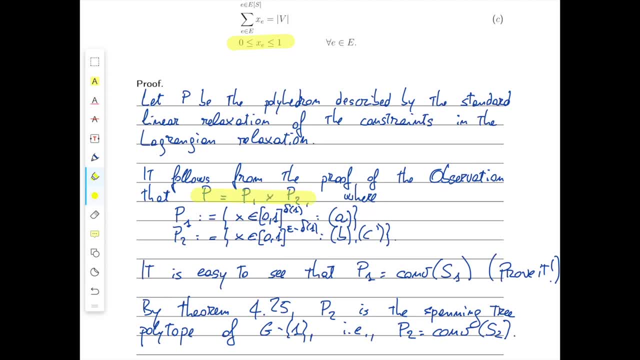 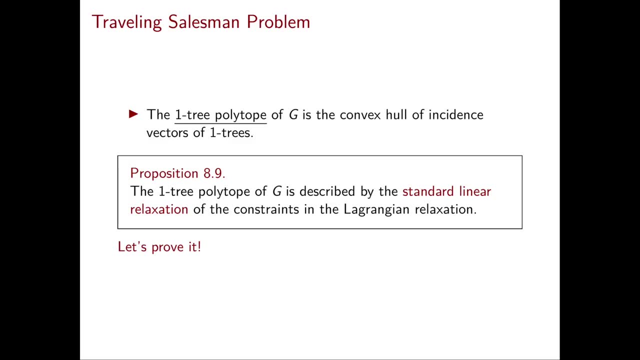 and so is their product P equal P1 times P2, and this concludes our proof. Let's go back to the slides. We've just shown that the one tree polytope of G is described by the standard linear relaxation of the constraints in the Lagrangian relaxation. 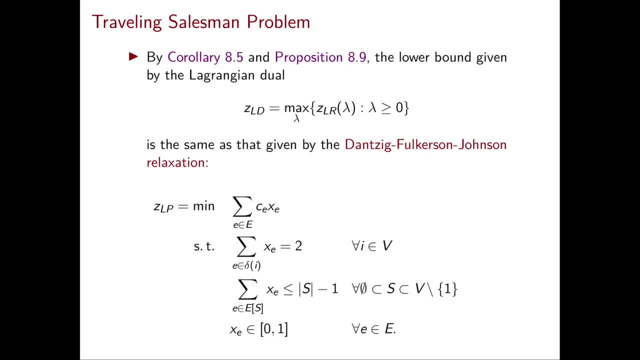 Therefore, together with our corollary 8.5, we now know that the bounds given by the Lagrangian dual so- ZLD, and the bound given by the dancing Fulkerson-Johnson linear relaxation, ZLP, coincide. Note that, as opposed to the general theory that we introduced in this chapter, where our original 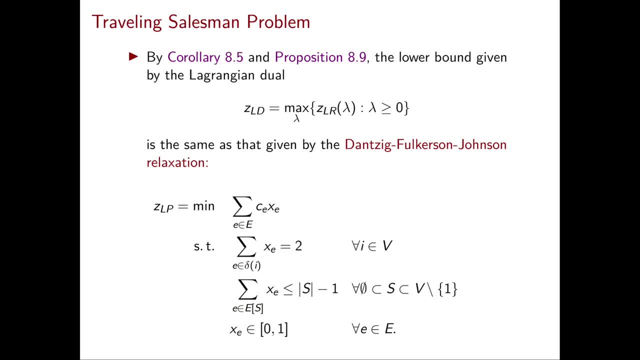 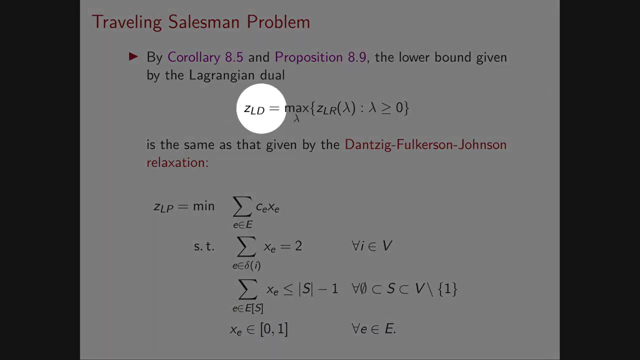 problem was a maximization problem. for our example of the traveling salesman problem, our objective is instead in minimization form. Therefore, all the bounds that we obtain are lower bounds and, in particular, the Lagrangian dual is defined to be the best lower bound. 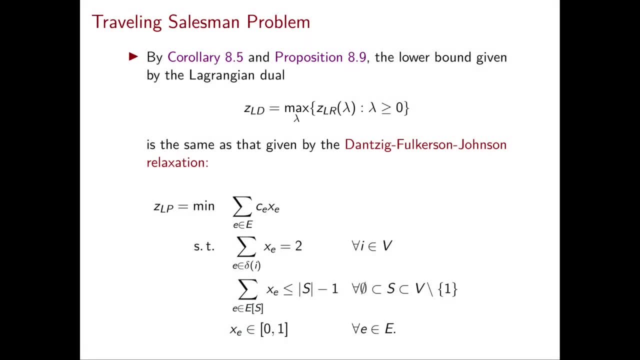 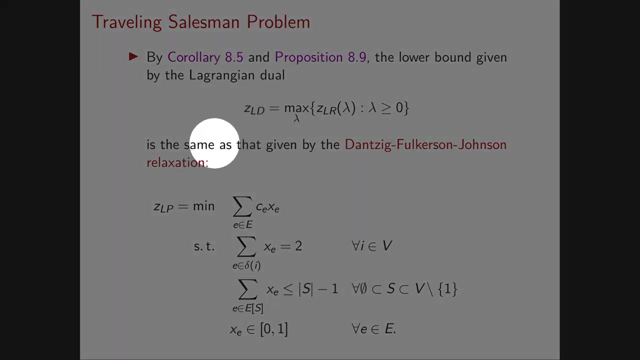 therefore we maximize over lambda instead of minimizing, as we did in the general theory. So essentially all max and min are just exchanged. In this case ZLD and ZLP coincide, where generally ZLD can be a better bound than ZLP. So in a sense this is a worst-case scenario for ZLD, because it's as weak as it can be. 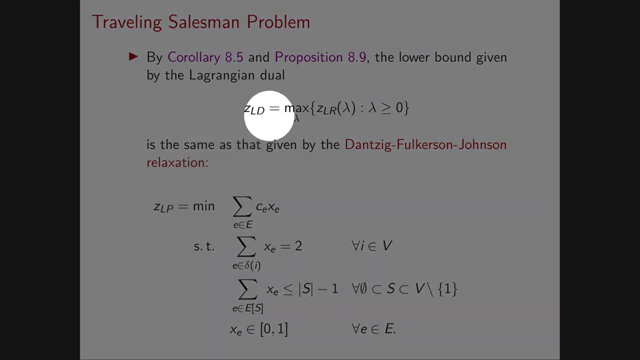 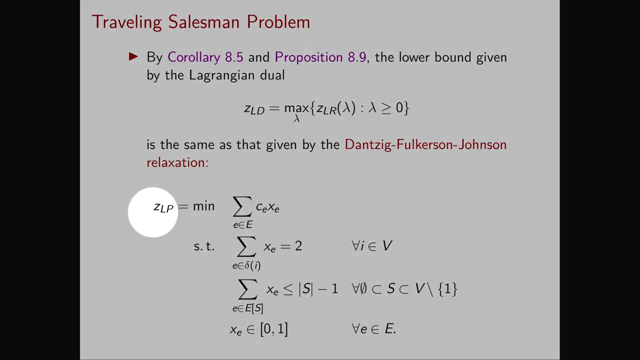 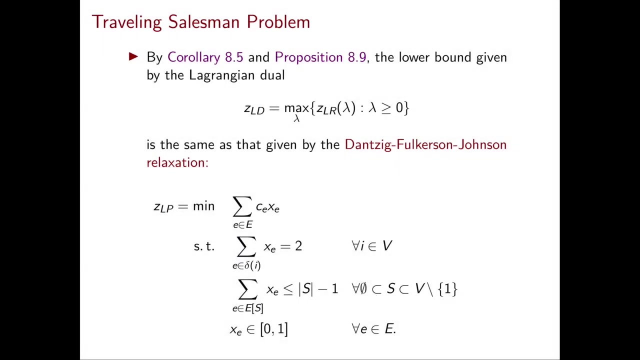 However, let's take a moment and discuss separately the Lagrangian dual and DLP to understand at this point the pros and cons of both these problems. So let's start by ZLP. So first, this is just a linear programming problem. however, it has an exponential number of constraints, and we know.